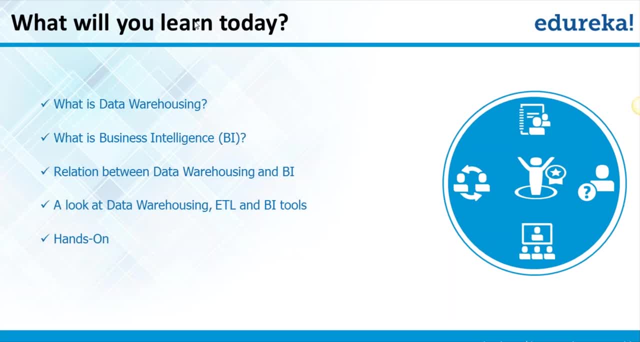 resource to attain this training? Yes, Vinay, so it all depends that in the current scenario or in the in the current age, everybody is going towards the data warehousing and business intelligence. so maybe, if you are from the mainframe technology or if there is someone from the mainframe technology, 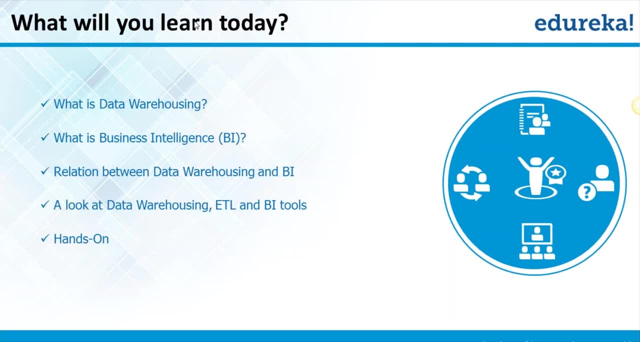 but it always makes sense to understand how the data flows into the data warehouse and how managers or the senior managers can take care of that data warehousing or data warehouse, which means that really the decisions based on the business intelligence system. so i would say yes and, most important, with 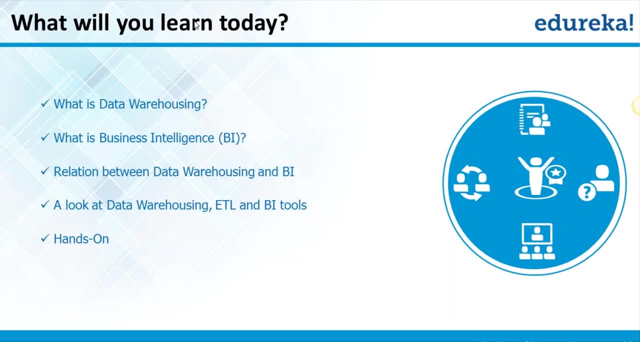 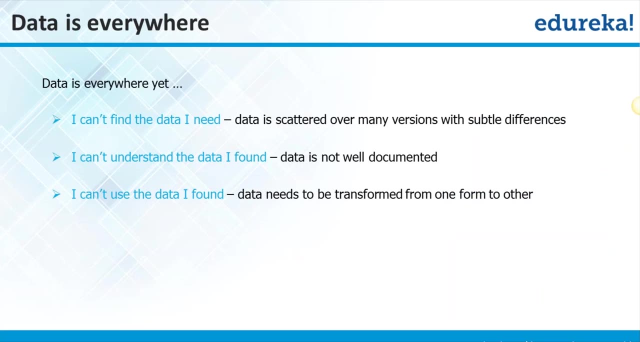 this particular course is that you do not require- uh, you do not require- too much of knowledge of this databases, and all because that all will be covered as part of the data warehouse and the data modeling in this course. okay, moving further. so, as i said, that data current age is: 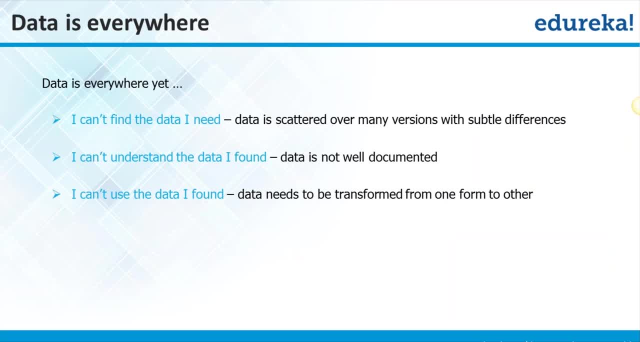 all about the data. data is everywhere. you might have heard about, uh, you might have heard this kind of questions that, uh, maybe from the, maybe from the ceo, cxos, or from the managers, senior managers or maybe team leads, that i can't find the data. what now data i need? right, because there are too many. 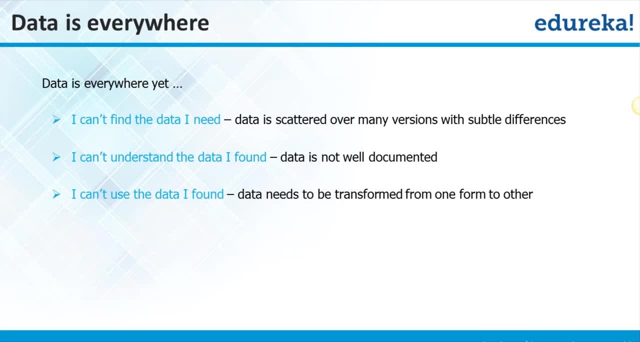 versions of data they are. they are data stored in different, different location. it could be just of your uh, it could be just your excel sheet, or it might be the data stored in the databases. so that is the problem. i can't understand the data i found data is not well documented, right. 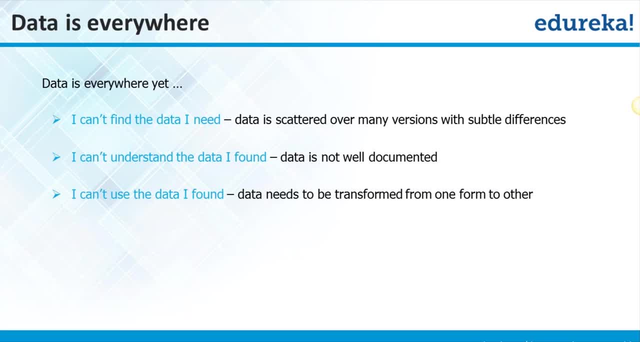 so, though, we have lot of data available with us, but we are not able to utilize that because we do not have knowledge about that data. we do not know what that data means. so that is the problem: i can't use the data i found data needs to be transformed from one form to the another. 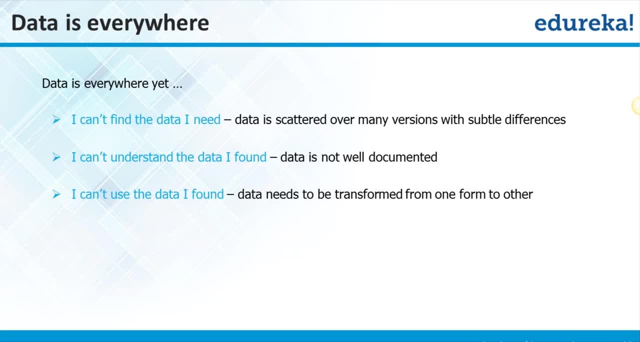 so, though, i understand what is this data, where it is stored, but i need to be uh, but data need to be in us in some synchronous form. right, i cannot have some data in the excel sheet and some data in the uh, in the xml, and if i want to generate some report or if i want to make 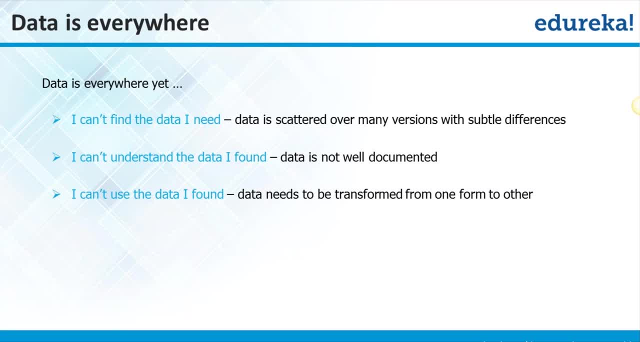 some, uh, meaningful decision out of that. that won't be possible, so either it need to be transformed into a, into a single form, or stored in a single format, so that is what is needed. so, even though we have data, we are not able to utilize that. and these are the. 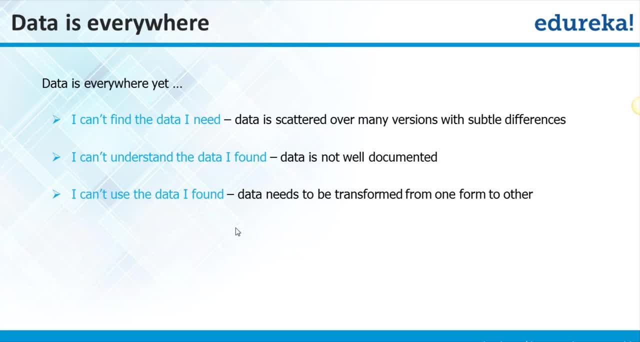 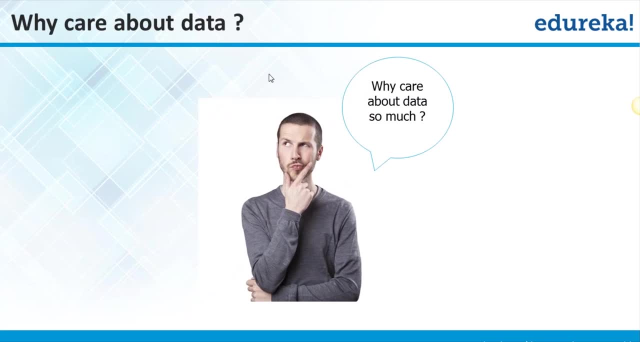 uh, couple of well-known reasons and i'm pretty sure that, uh, you might have heard or you might have come across this in day-to-day scenario. so it is not just about the data warehouse or database, it is almost everywhere. so why to care about data? as i said that we are talking, 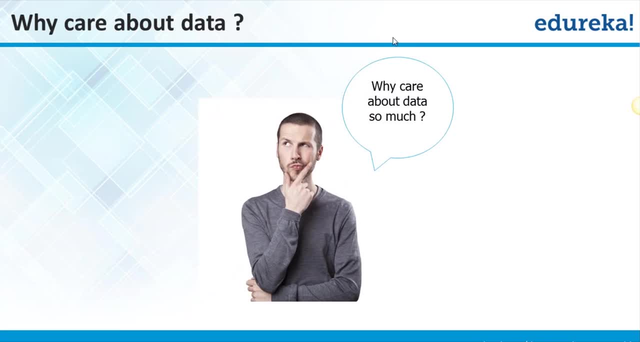 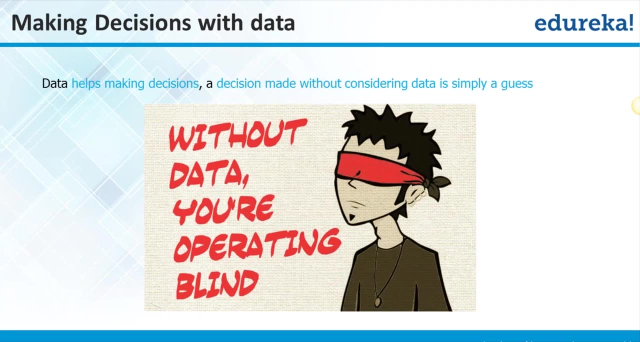 about this data warehouse keeping a lot of data. so why we are worrying about the data? right, because without data you cannot make any decision. this, So it's true for your data warehousing system, for your business intelligence system, or maybe in your day-to-day operations. 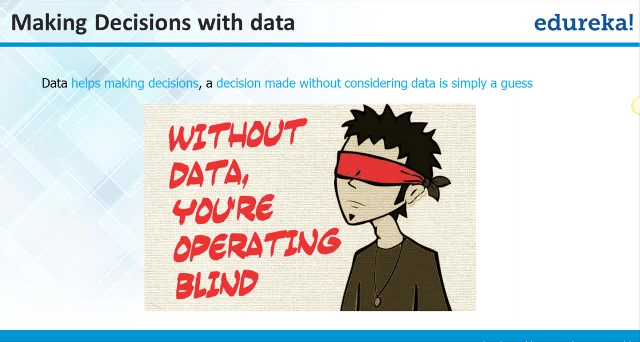 You need some data to make a good decision. Data helps making decisions. A decision made without considering data is simply a guess, And I believe that everyone will agree to this. that sorry, sorry to stop over here. Mohan says that I am not audible. 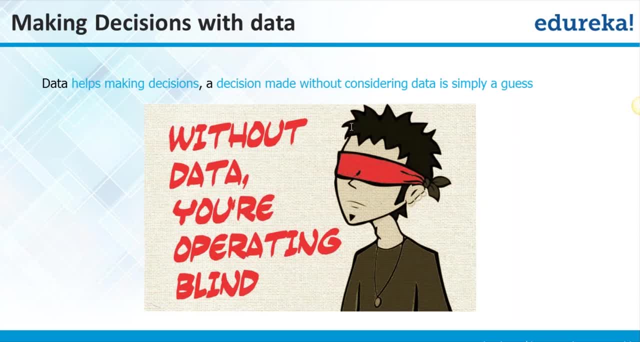 Is that the case with others as well? Can I get quick response? No, Mohan, others can hear me properly. I think there is some problem with the audio at your end or maybe you need to join again. I'm not very sure, because I got a couple of responses and everybody says that they. 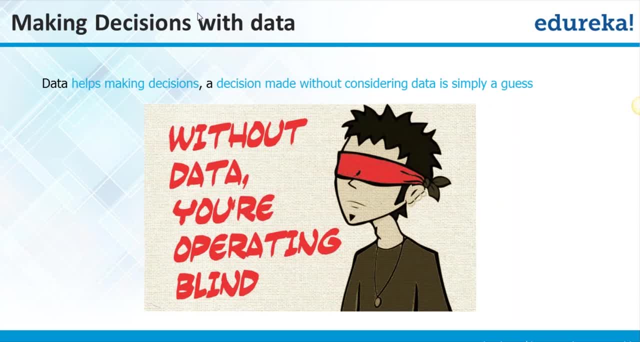 can hear me, So I'll continue. Probably you can join again. Okay, Thank you. So making decisions with data. So if you're not considering the data and if you're making some decision, that is more of a guess, That is more on your past experience. 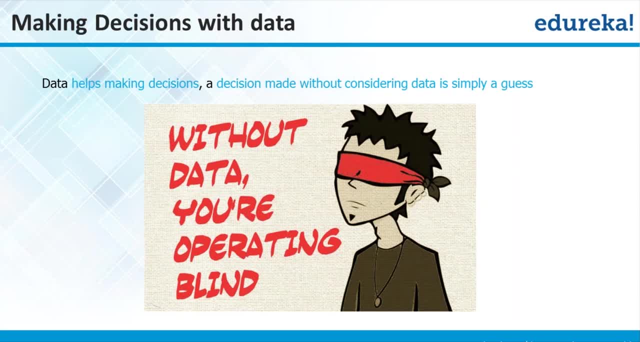 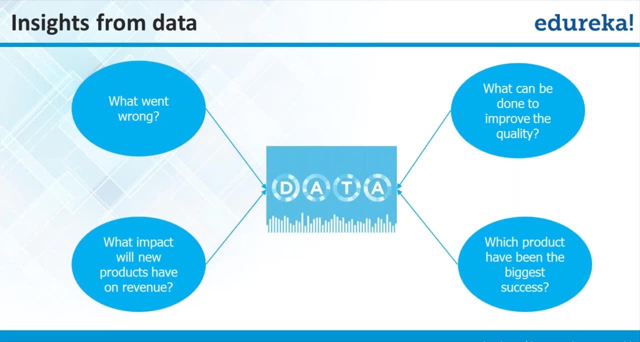 But when you are looking at the data, then you are able to make a correct decision, right. So what insights that we can get from data, And this slide explains it very well. that may it be about the quality, may it be about 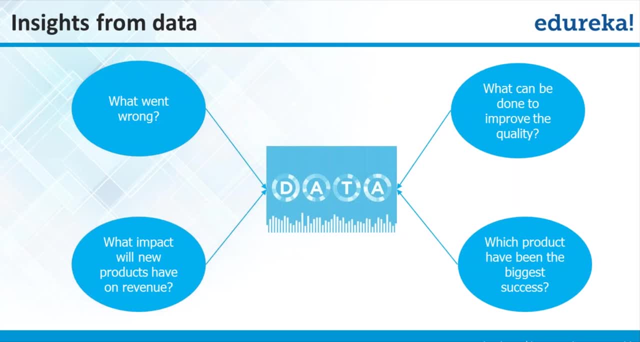 the success of a product. So how is it worth it? how about the amount of growth, Whether it's the product or the revenue, Whatever is the overall cost or the overallróno of the product or the amount of revenue About what went wrong. 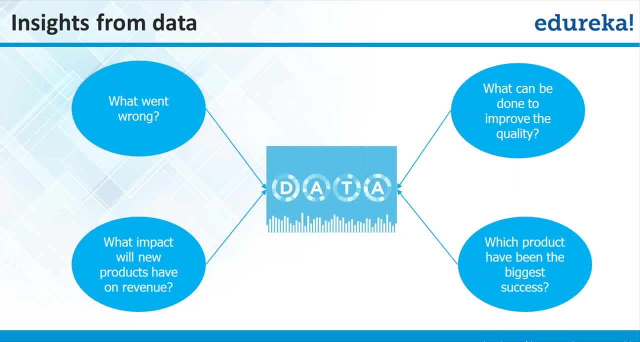 What went good About the future plans? Everything can be done with data. So, if I have my data available and believe me that every system or every organization is maintaining data, It is all about how you are utilizing data. So, if you have your data accurately organized or if you're utilizing your data correctly, 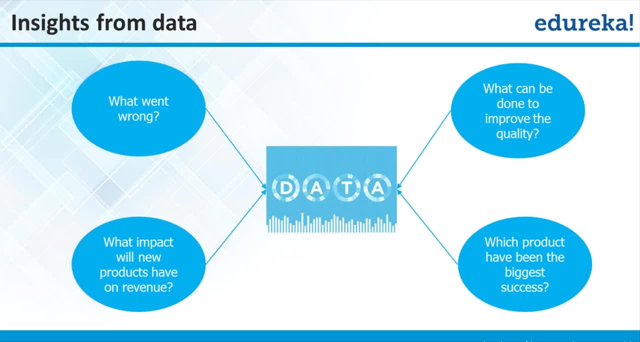 then you can answer this question: What can be done to improve the quality Outs謝king? So maybe you can have the KPI matrices, you can have the fault ratio, order ratio, those kind of things. Which product have been the biggest success? 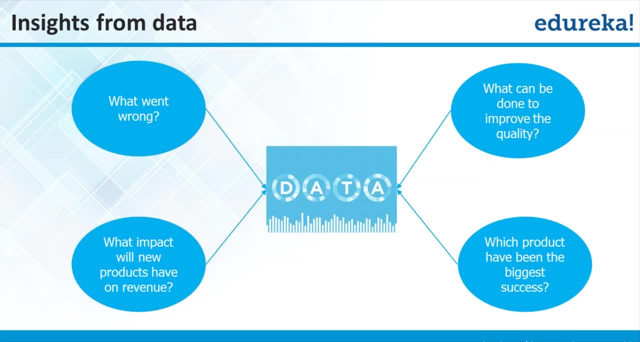 So if you have seen in the market today that in the marketing team, or with the product launch, or with the discount offers, all this is data driven- right, They are giving discounts almost every day, almost every weekend, right, That is all on the data that they see, right? 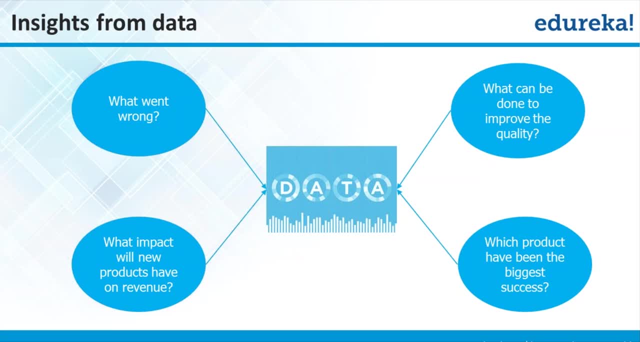 So people are buying something on the weekends so we can give discounts on other things, on the related things, those kind of things. So all this is driven by data. What impact will new products have on revenue? So if I talk about this in the telecom industry, you can see that there are many plans coming. 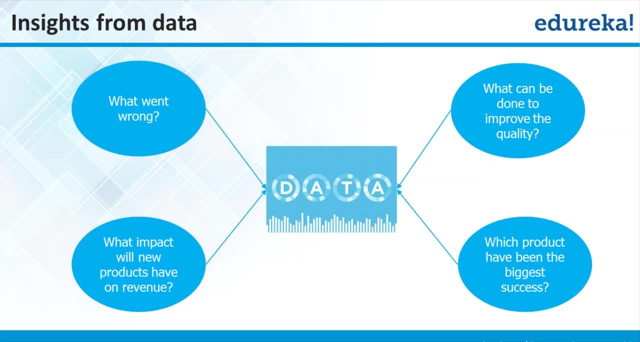 these days right. So every month, every fortnight, they are changing their plans. why? Because they have data To make those decisions. Earlier, it used to be just a single plan or a couple of plans available with a telecom provider. 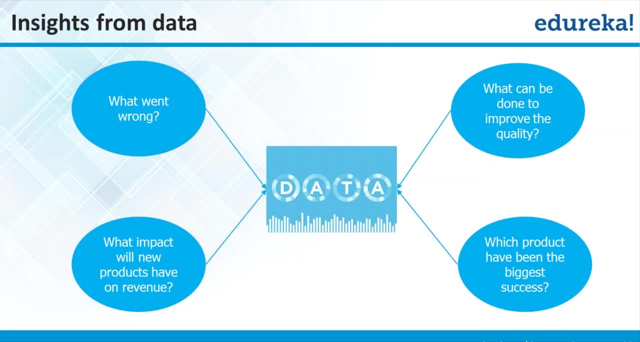 Now they are providing offers almost every month, or maybe more frequently. That is all depending on the data and what went wrong. So even when you are considering the data, maybe sometimes your things would not click, or maybe if something went wrong previously that you can find out with the data. 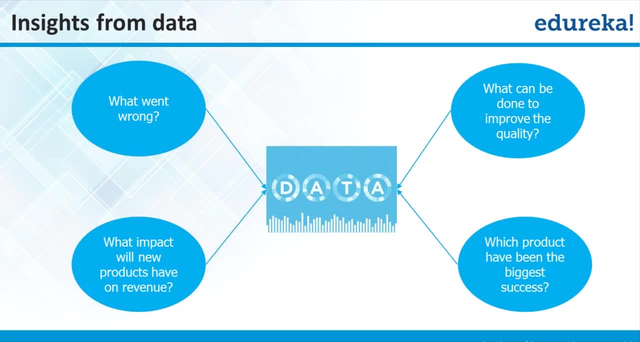 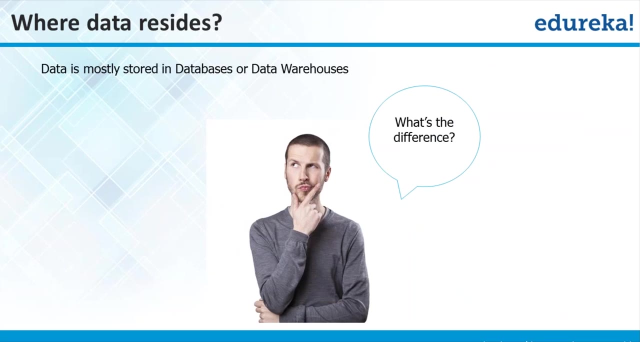 So maybe you targeted wrong. Maybe you targeted wrong geography. may be you targeted wrong audience. So all those things can be found out using data that you have available in your system. Okay, So where does data reside? So data resides mostly in the databases or data warehouses, right? 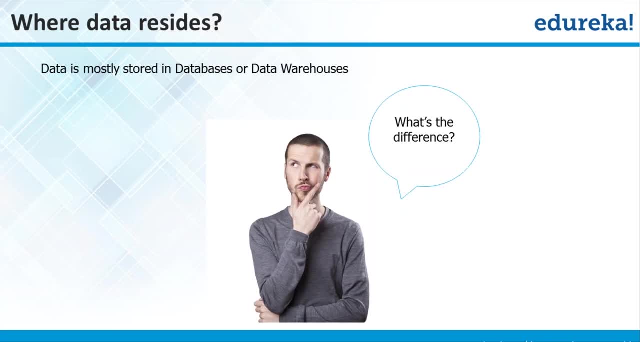 And when I say databases, it could be your relational database. it could be your relational databases like Oracle, MySQL, MSXs. It could be your unstructured databases databases. it could be in your excel sheet, it could be in your text files. it could be. 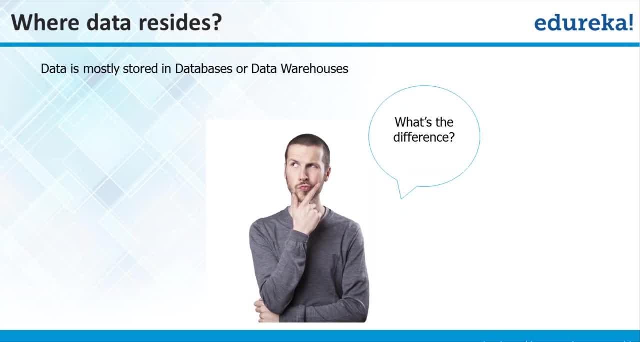 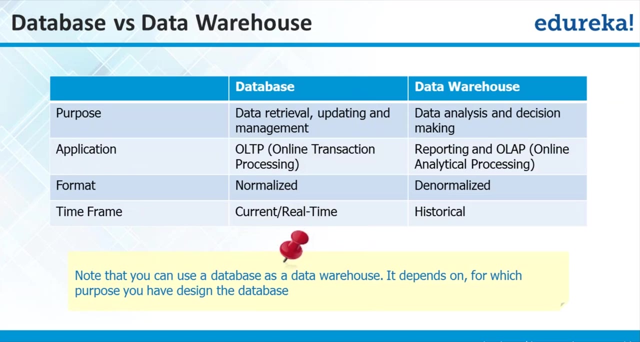 in your log files, everywhere data resides, and similarly we call it as a database, and a bigger picture of this will come into our data warehouse. So we have this question almost every time. so what's the difference between databases and data warehouse? So, to make it simple, we have this table to differentiate between the database and data. 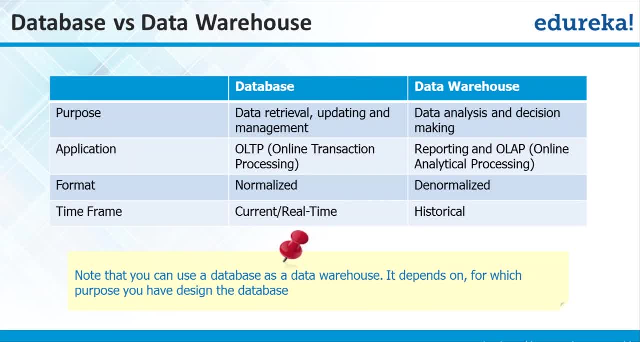 warehouse. but normally when I classify this database in a data warehouse, I say something as a customer facing application or online transaction processing system. So that is driving your business. So if you talk about this superstore database, some database that you are using for billing- 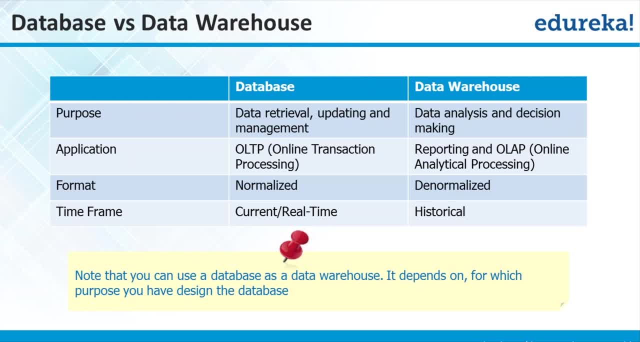 your clients. If you talk about this telecom system, if you talk about this banking application, maybe the internet application, this is your database, Or where you are maintaining your record, whereas data warehouse is more of a OLAP database, that is, online analytical processing that is used for analysis purposes. that will hold. 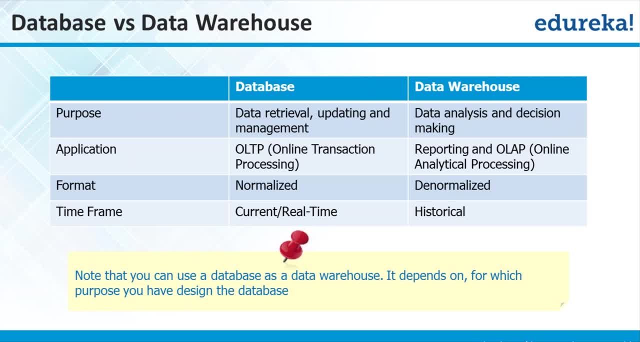 data for a longer period of time. that will store history of data, So I will go through this. when I talk about database, the main purpose is data retrieval, updating and management, whereas data warehouse is about data analysis and decision making. So when I talk about my database, 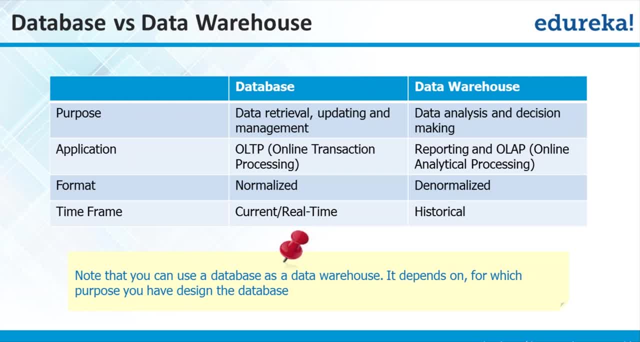 My major aim, or my main aim, is to get the data fast. I can update data quickly. I can see my data. that is what is required out of a database, whereas data warehouse is completely used for the data analysis and the decision. So might be your data retrieval is taking bit long. that is fine. 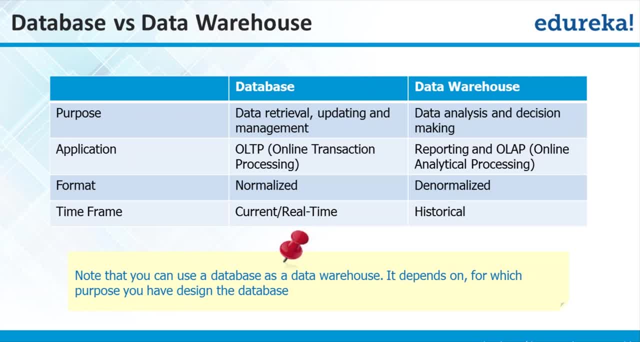 Normally you do not update your data in your data warehouse. You only keep on inserting data. and when I say that you do not update, that means user cannot update the data. Maybe you have your batch process, maybe you have your ETL process to update your data warehouse. 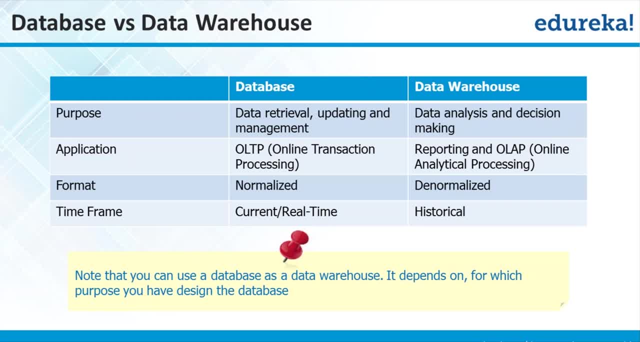 Application. wise, as I said, that database is classified as OLTP, that is, online transaction processing, whereas data warehouse is classified as reporting and OLAP, that is, online analytical processing. In the database, you store data in to the normalized form, whereas in the data warehouse, you store it into a denormalized form. 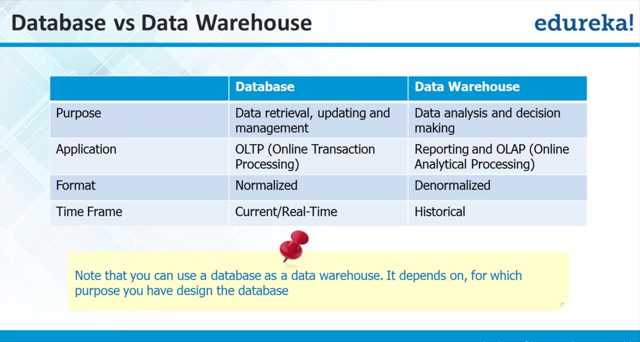 Again, this normalized and denormalized itself is a very big topic to discuss over here. but in short, when I say that it should be in a normalized way, that is, data retrieval or updation is very fast with the normalized database, whereas with the data warehouse it is more. 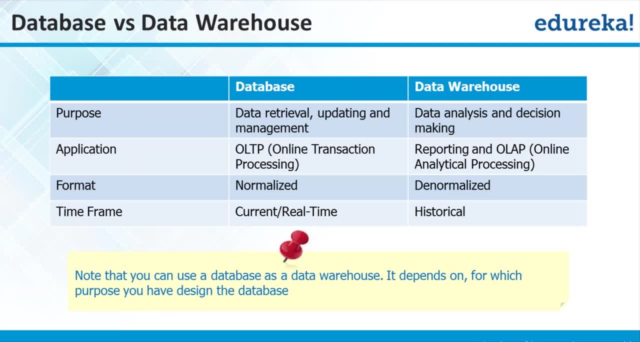 about the data retrieval: Data retrieval as in for the particular region for a particular product. So you have more number of columns in a single table so that your data retrieval or your reporting becomes very easy with the data warehouse format. Again, as I said, that this is just a high level overview. 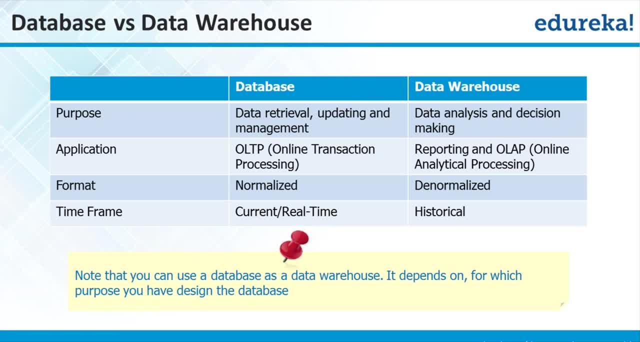 This itself is a very big topic, but when we talk about the time frame, database is more of a current or a real time thing, whereas data warehouse is mostly a historical data that you are capturing into the data warehouse Again. Having said that, Note that you can use a database as a data warehouse. 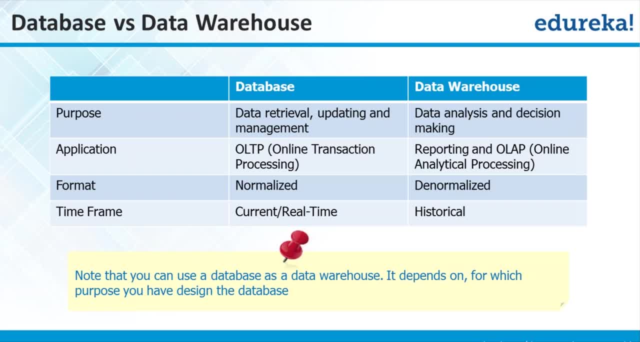 So, with certain enterprises, with certain application, you might see that they are calling your database as a data warehouse because they are storing data for a year, for five years, into a same database and the same database is being used by the real time application, by the users and by the analyst as well for doing the historical analysis. 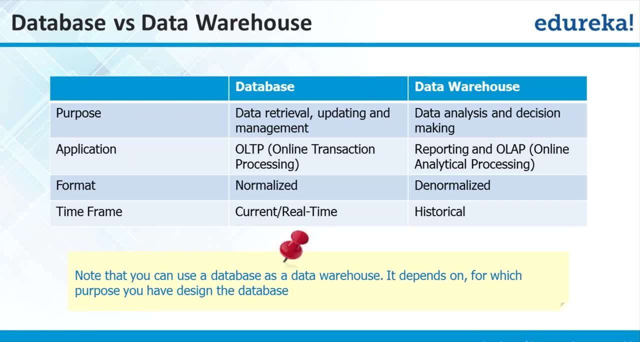 Again, it depends on for which purpose you have designed the databases. So Yeah, That is also one of the approach that you are using only your database for both the purposes. Normally, in database we retrieve and update through programs. How about? how about data warehousing? 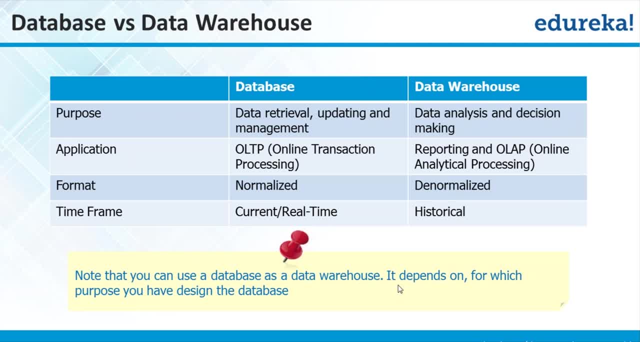 Can you elaborate on the data analysis? Okay, So in database we update. we update data with the user, with the user activity. So when I say that a database may be in the superstore database or maybe in the In case of programs as well, in case of telecom database, 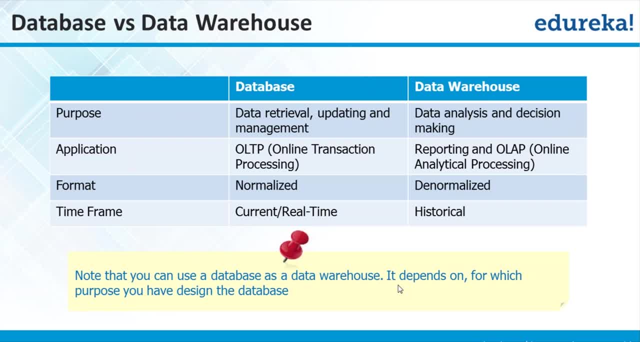 So maybe you are making a call that will be logged in into the database as part of the, as part of some program, whereas in the stores, whereas in the superstore database, if you are making a purchase that would be entered by a cashier, to store that into a database. 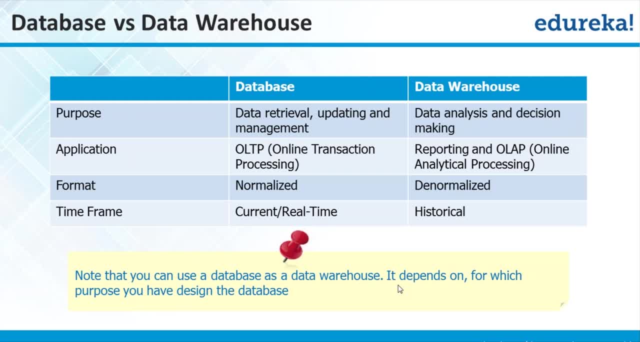 whereas in data warehouse you store data which is available in your data database as well as with the other other third party databases. So, To take an example, in my superstore or in my particular, any detail store, I would be needing data only for one month. because, for because during only one month I'm allowing 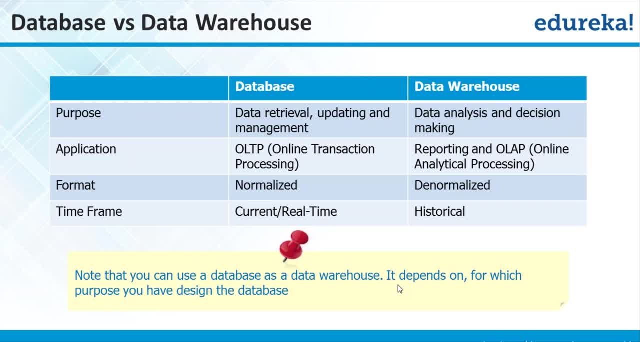 return for that that product? Okay, So I want to keep a data for one month into my system so that I can find that bill, I can do a return, I can do a replace or whatever. Okay, I may not be interested in data which is older. 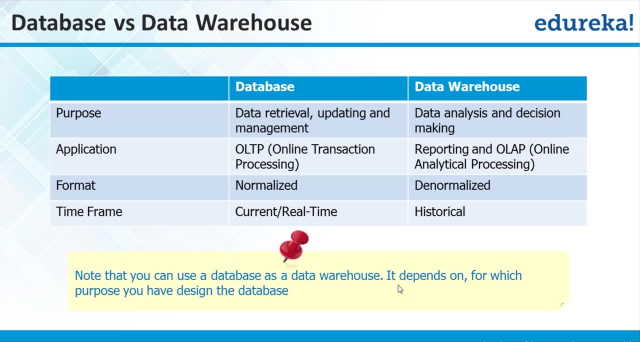 So then, one and a half month or two months, right, That is enough for my, for my purpose. So, I would be keeping only one month, or maximum two months, of data into my database, and whereas I would be purging all the data before that. 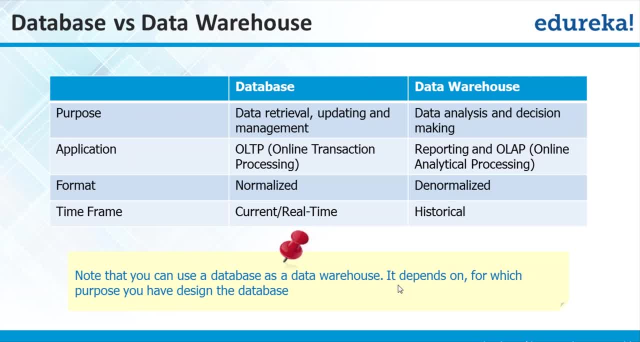 And when I say that purging, you cannot push that right away. So basically, what, what enterprise or what organization before is that moving that into a separate database and that we call it as a data warehouse? So there is no point is that you are storing data as is into the database? 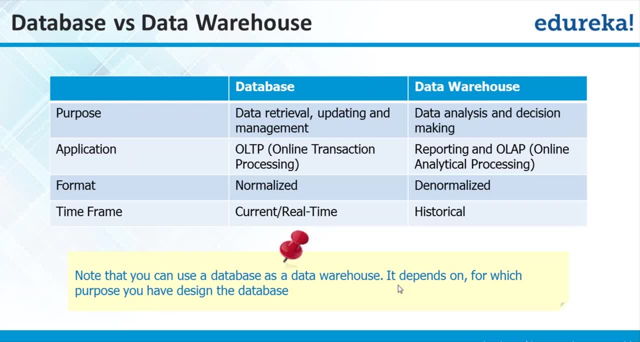 Okay, Okay, So you can store it into another database into the same format. there You do certain kind of transformations, there do certain kind of denormalization, and then you store into your data warehouse, so that in data warehouse you might be having a historical. 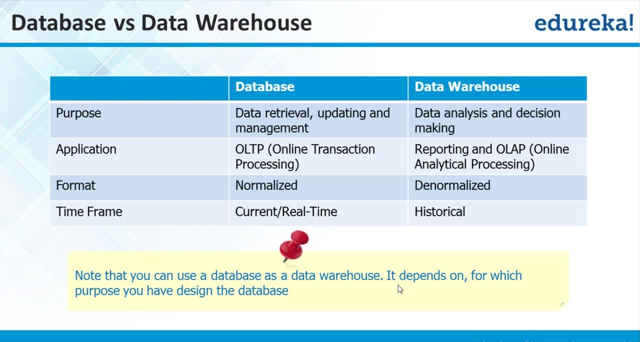 data of five years, 10 years or whatever period that you want. Another thing is that when I talk about the data analysis- so when I have data for around five years or for around three years- I can take a decision quickly. Okay, For this particular product. it worked well during this particular festive seasons. it. 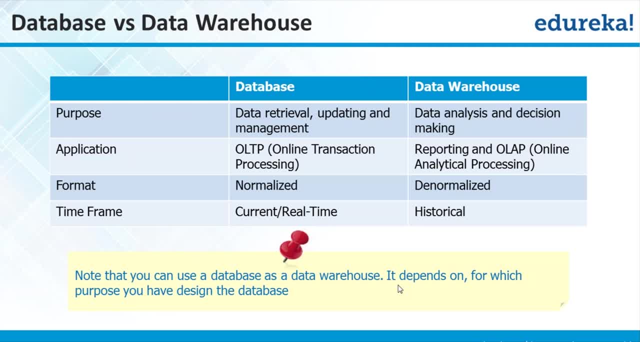 worked well during the monsoon season and that way I can. I can provide offers, I can do revenue analysis, I can do quality analysis. all those analysis can be done based on the data available in the data warehouse, and all this data is normally loaded through a ETL. 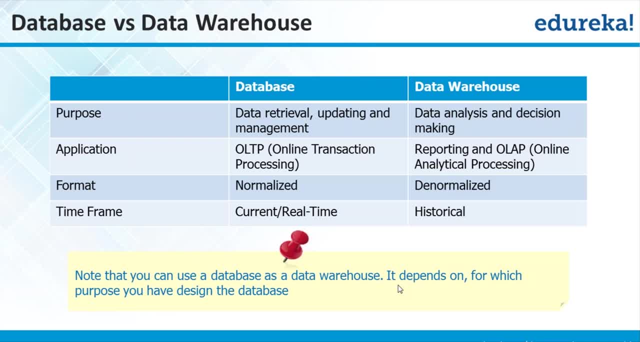 process. I hope that answers your question how often data from a database is moved to a data warehouse. So it is again depending upon your design, Some people. Some people do it Okay, Some people do it in real time. that is every 15 minutes, every 20 minutes. 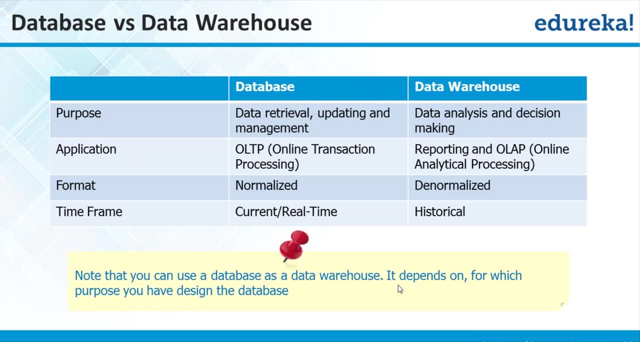 Some, most of the places, it is overnight data refresh, that during the night, when you do not have any any major user activity, you you load your data from database to a data warehouse. It could be weekly process, it could be monthly process, depending upon the data that you have. 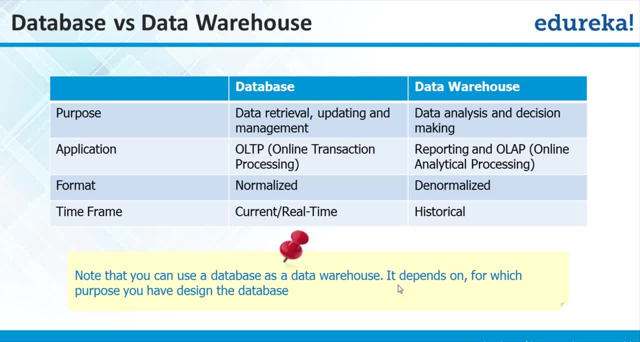 depending upon the domain that you that you are working on or what kind of analysis that you want to do. What's the size of data that we can store in warehouse? Is there any limitation? No winner. There is no limitation that the amount of data that you can store in your data warehouse. 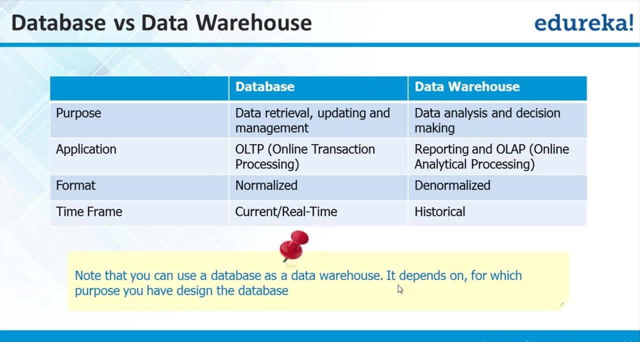 It could be up to. it could be up to multiple or hundred or thousand of TBS. It could be in a few hundred of GBs. It completely depends upon your requirement or the data that you have available with your organization, Okay, But again, with the data that you have, you need to decide that which kind of database? 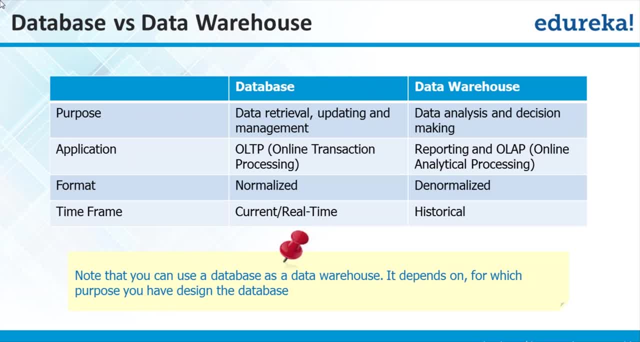 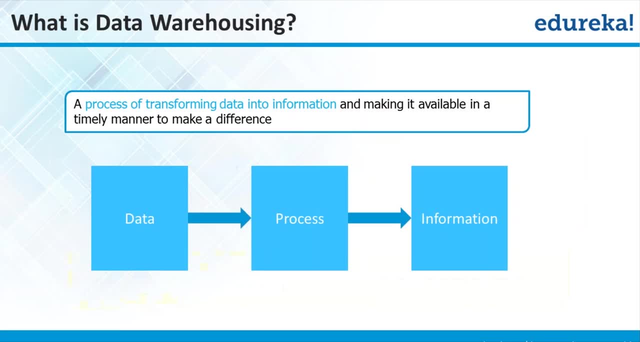 Okay That, which kind of database would be good for you, which kind of data warehouse would be good for you? or if you have very less data, then probably you can use databases, your data warehouse, those kind of things. Okay, so coming back, what is data warehousing? a process of transforming data into information. 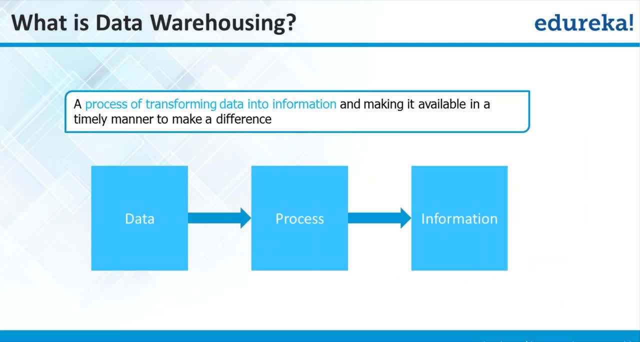 and making it available in a timely manner to make a difference. Okay, so we have data available in our database, But probably when you ask some analysts to analyze on the data, it would not be very helpful because you would be storing product information at one place, sales information at one place. 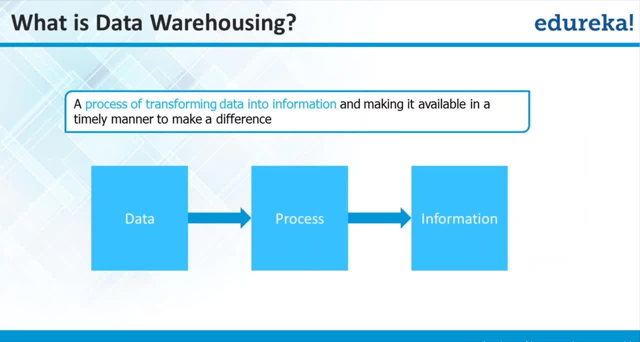 or revenue information at one place, to store that data or transform the data and store and to make a meaningful information out of that. That is the purpose of data warehousing. Okay, So you have your database data available in your database, You process the data and you convert that into information. 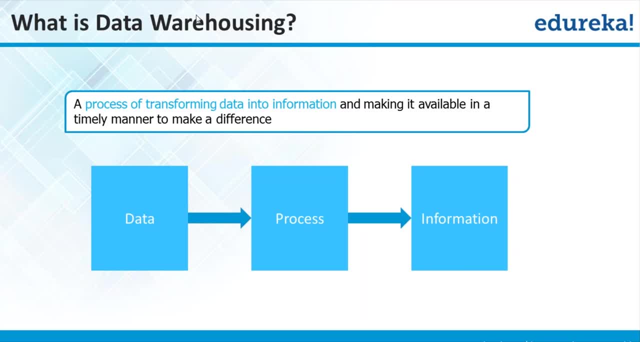 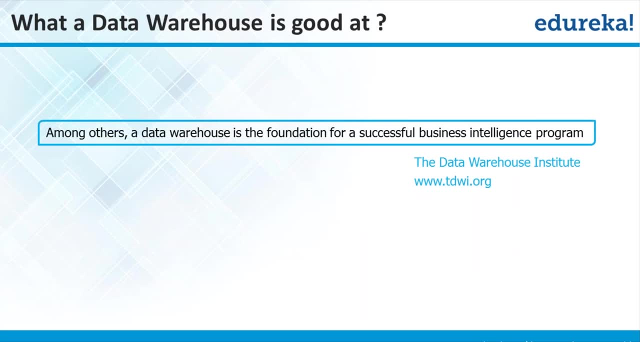 That is the purpose of your data warehouse. again, in the data warehouse They are two Data warehouse guru, that is, Inman and Kimball. They have their approach and that is again a very detailed topic, But there is a high level overview of the data warehouse. 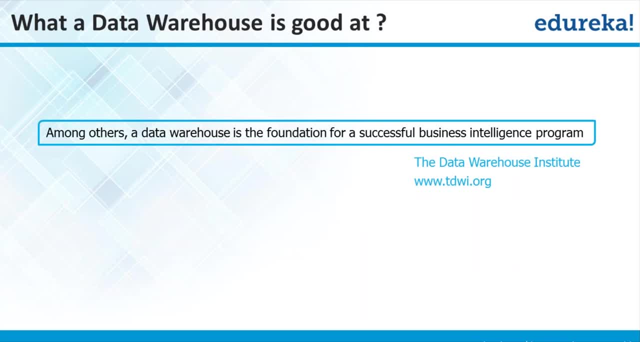 Among others. a data warehouse is the foundation for a successful business intelligence program. This is again given by the Data Warehouse Institute that is TDWI. That data warehouse puts a foundation for a business intelligence program. Okay, so that you can intelligently use that data. 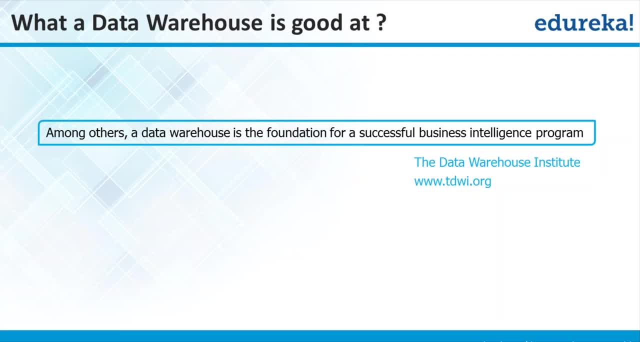 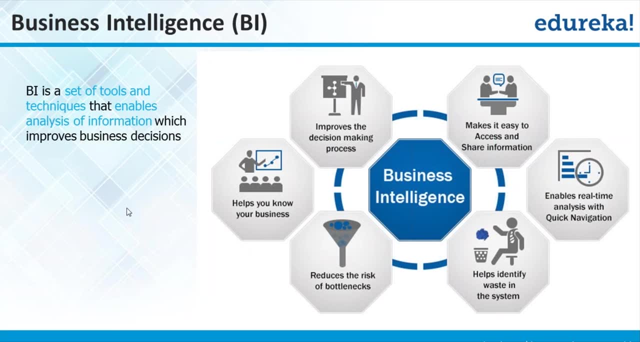 To drive your business decisions. That is the purpose of your data warehouse. Now coming to the business intelligence part of it. So when when I talked about this data warehouse, it was all about keeping the data. Now when I talk about the business intelligence, 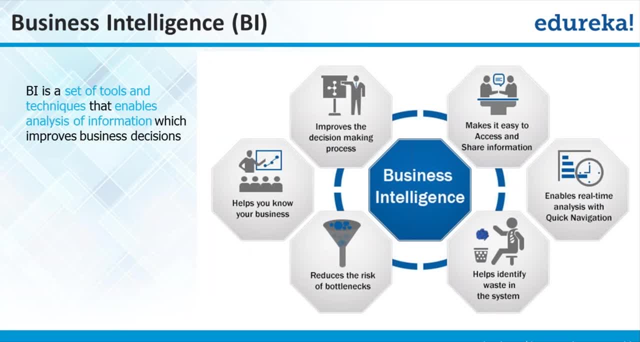 So BI is the acronym for that. BI is a set of tools and techniques that enables analysis of information which improves business decisions. Okay, So we have all this data available. Now we need to have certain kind of tools and techniques through which we can analyze. 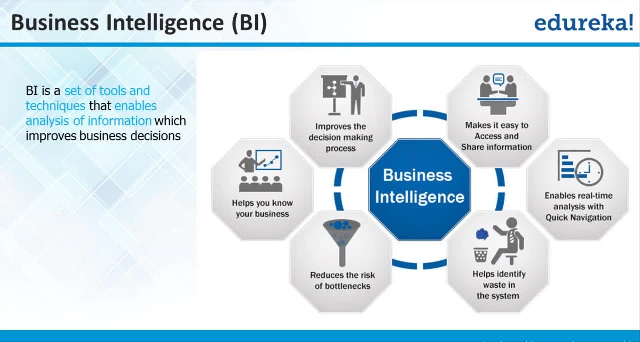 through which we can do the analysis of this information, And that is a part of BI. There are various things that we can do with BI and, to name a few, we have this in slide, So BI makes it easy to access and share information. 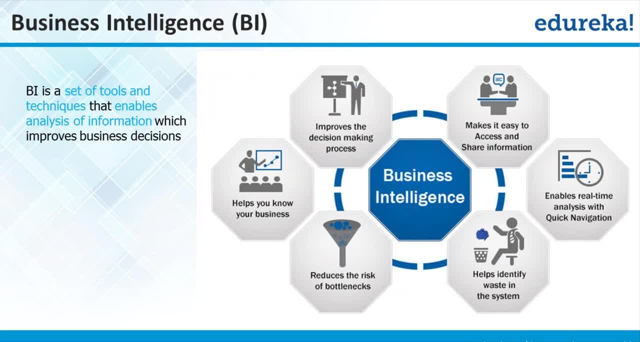 BI enables real time analysis with quick navigation. BI helps identify waste in the system. BI reduces the risk of bottlenecks, improves the decision making process, helps you to know your business. Okay, so again, when I say that we have information in data warehouse, now let's say: you have information. 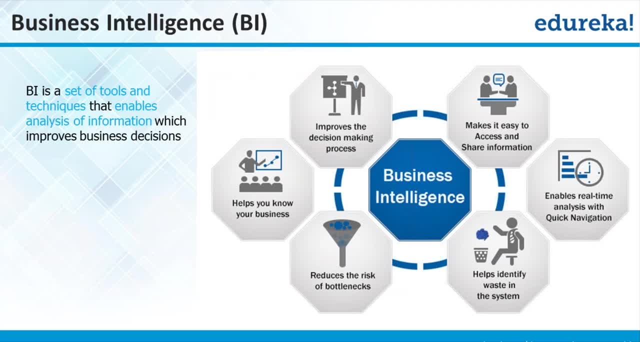 of 1 TB in your data warehouse. Now it's up to you that- how you can make an effective use of that information. and that is a part of BI. That are a business intelligence, Business intelligence tools are business intelligence techniques. that how you can make. 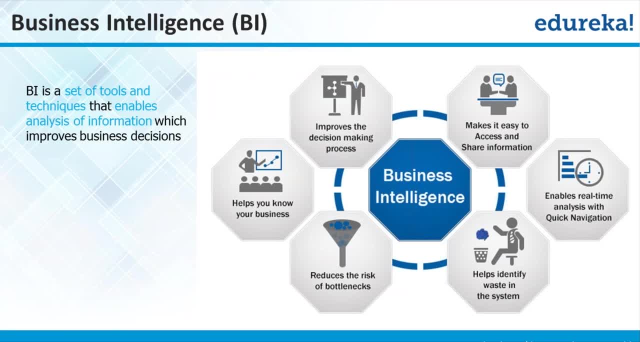 a business decision: how you can remove the waste product or remove some of the product which is not doing good, which is giving you loss, which region is more profitable, which product is best selling in the market, those kind of things, Or what all changes that you can do in your organization that will increase the revenue. 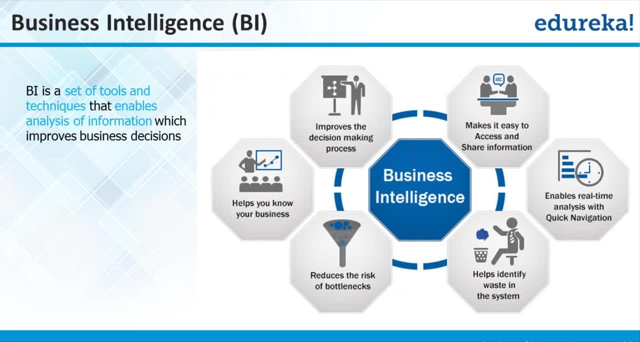 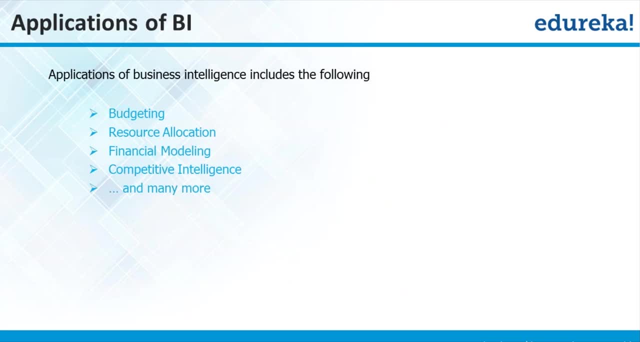 that will increase the employee satisfaction, those kind of things, Or customer satisfaction. All these are part of BI. So when I talk about the application of BI again, it can be done for the budgeting, resource allocation, financial modeling, competitive intelligence, predictive analysis, everything. 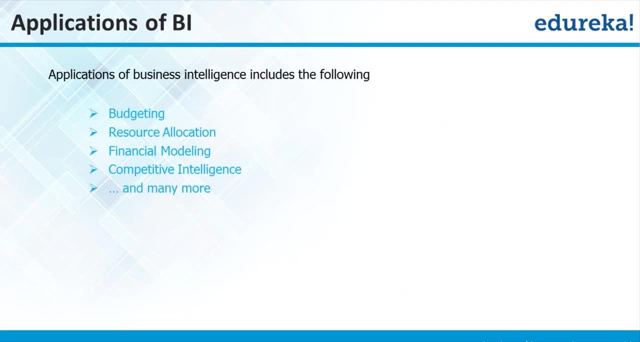 You can do this business intelligence, So you have your data available for, let's say, historic data for 2 years, 5 years. Based on that, only you can do your budgeting Right. Based on that, only you can do your forecasting. 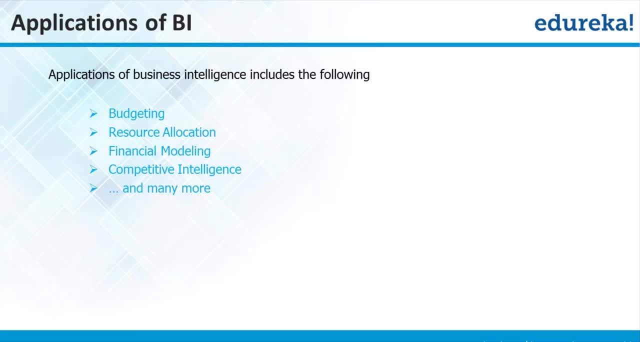 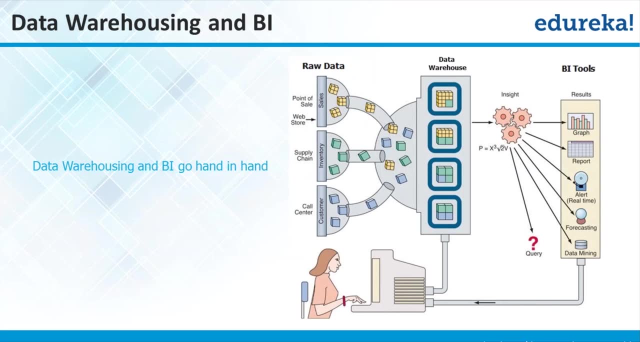 So it need to have some kind of data and some kind of tools and techniques so that you can derive information out of that. And when I talk about or what is this course is all about data warehousing and business intelligence. So why we are targeting two things. 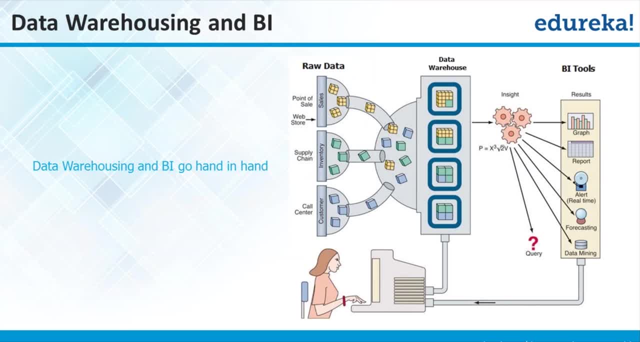 Because both of these things go hand in hand. Okay, When I want to do a BI, I need to have certain kind of data warehouse. Having said that, we can do a reporting. We can do a reporting on databases as well, or on a smaller set of data as well. 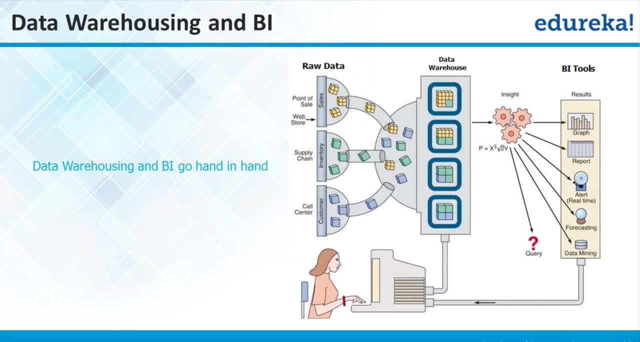 But in the current scenario, when we are talking about the big enterprises, big organizations, they all have a data warehouse, And to utilize the data of your data warehouse you need to have a BI capabilities. Then only there is a point of maintaining a data warehouse. 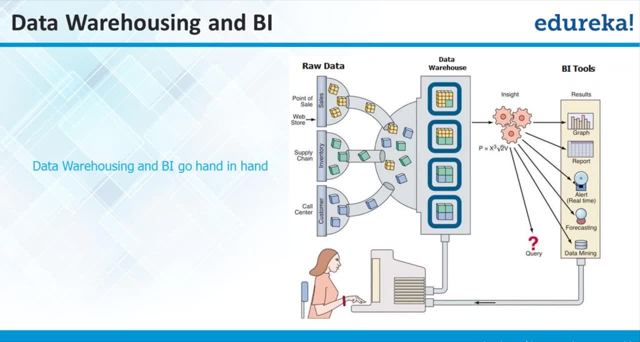 That's the way you can utilize your data warehouse. Okay, So, if I go through this architecture, Okay, Okay, Okay. So, if you want to do this, you need to have different kind of raw data. It could be from the different LOBs. 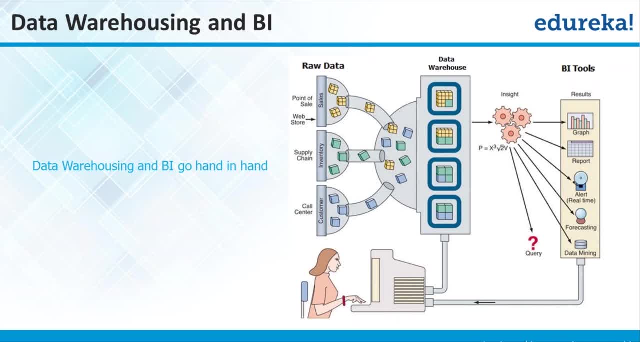 It could be from the sales team, It could be from the inventory, from the customer, from the HR that you would be having, that you would be getting your data. To transform all that data into a single format And then you installed it into a data warehouse. 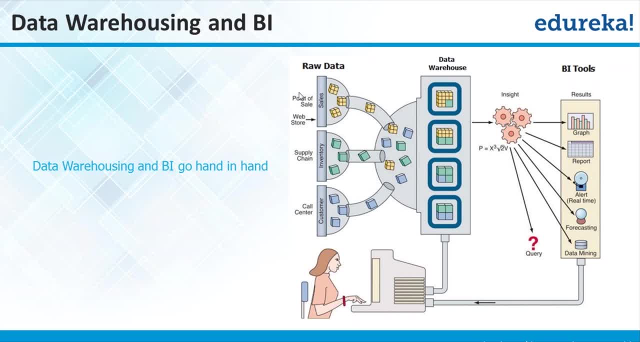 So maybe in the customer location you might be having data in a different format. In the supply, in the inventory you might be having data in the different format monthly level. someplace you would be doing at the weekly level. so you need to do that aggregation, you need to do that transformation so that data is at same. 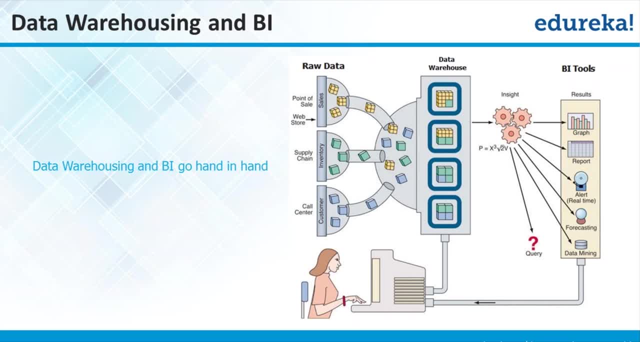 level data is clear so that you can do analysis on top of that. so once you store your data into your data warehouse, after that you can generate your, you can generate your reports out of that and those reports could be into the, into the graphical format, tabular format. that could be a plain, plain queries on onto. 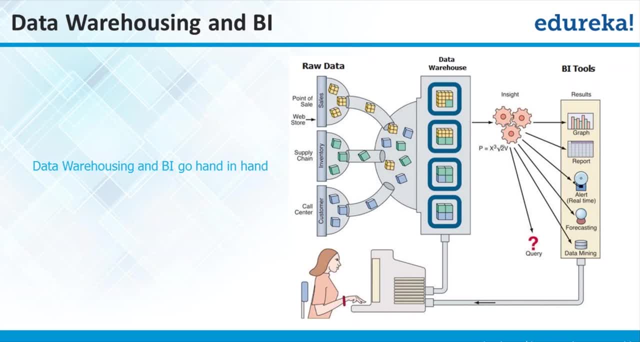 the data so that you can retrieve some data, you can do a budgeting, forecasting everything out of that data. okay, so there is a question that why can't database is stored? stored historical data. the reason why we don't prefer storing historical data into a database is because if that will increase the 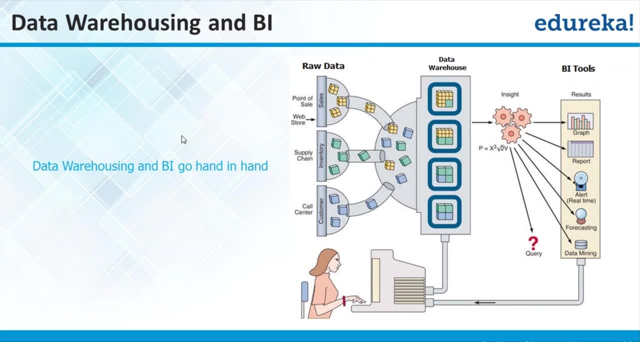 size of your database. okay, so right now I want to is to. I am only interested in two months of data for my superstore database or for my retail database, But if I'm trying to store data for last three years or for six years into my database, 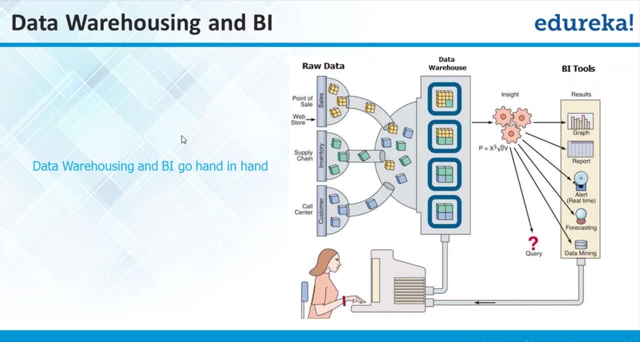 then that would definitely hit my customers. When I'm trying to retrieve, insert, update or select any record, that will take more time because I'm hitting maybe 20 times the more volume, 50 times the more volume and that's the reason. 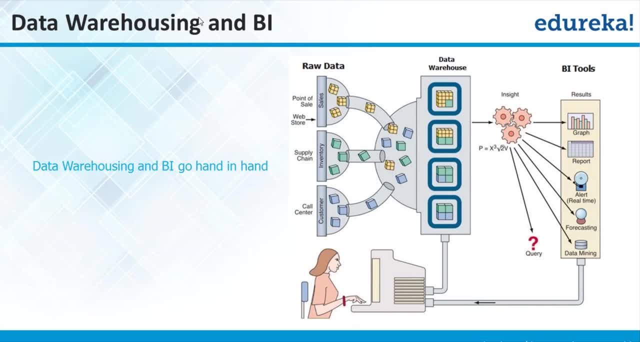 So it is more for the performance and the maintenance perspective. So what is the exact difference between the data warehouse and business intelligence? This is the question. So data warehouse is all about storing your data, storing your historical data, whereas business intelligence is the tool and technique. 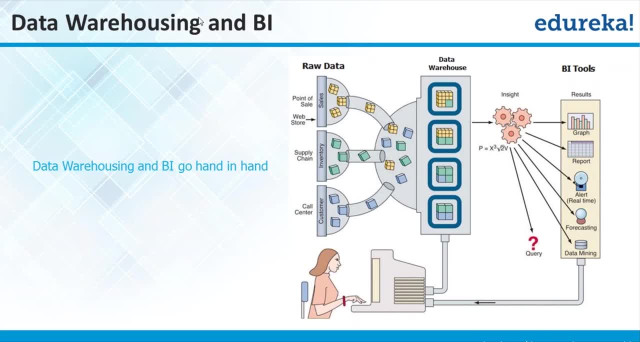 with which you can utilize that data stored in your data warehouse and make a business decision out of it. I hope that makes sense. What are the techniques to store? there's another question: what are the techniques to store the raw data into data warehouse? 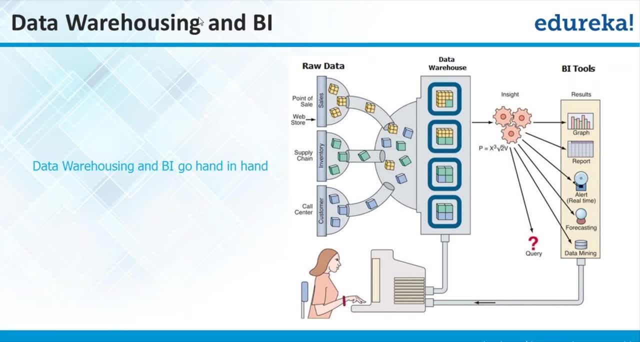 And the technique to store raw data into your data warehouse is the ETL, that is, extract, transform and load. So in that process you might be having multiple set of raw data or structured data, unstructured data. Then you transform that into a single format. 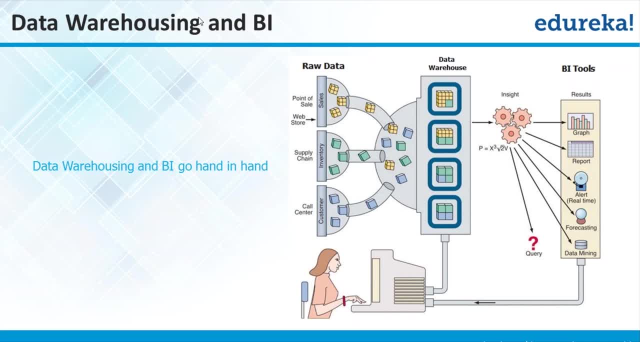 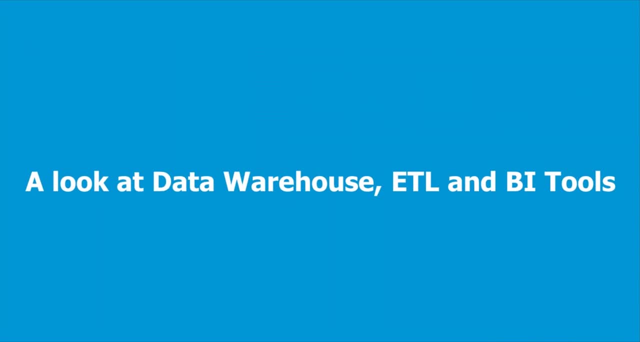 or into the required format, and then you load into your data warehouse And this process is known as ETL: extract, transform and load. This usage of BI mandatory along with the data warehouse? don't we have a reporting techniques within data warehouse? 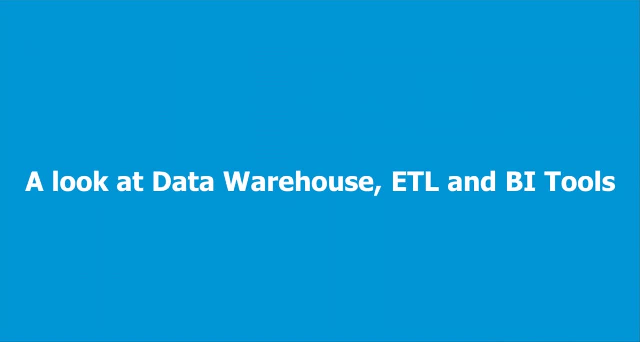 So when we talk about this, do we have a reporting capability within a data warehouse? Then it is more that we are talking about the products that are available in the market. So, yes, there are certain products which comes as a combined package, where you get 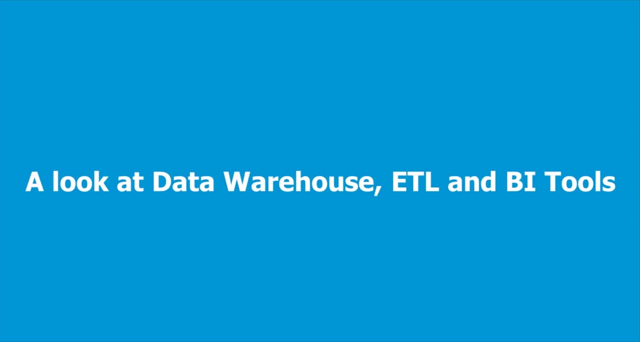 ETL package. you get a database, you get a data warehouse and you get a BI capability, but broadly speaking, these are two separate terms. Data warehouse is more about storing data. BI is more about using that data. You can have a single tool available. 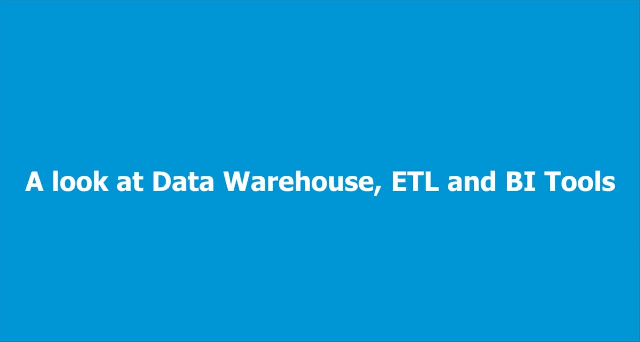 to use that information, to store the data and to analyze that data. Probably you might have some vendor which is giving you a database and giving you tools as well so that you can utilize that data, But broadly speaking, these are two separate items. We can track that data, use that data, do it and get it done as soon as it's possible. 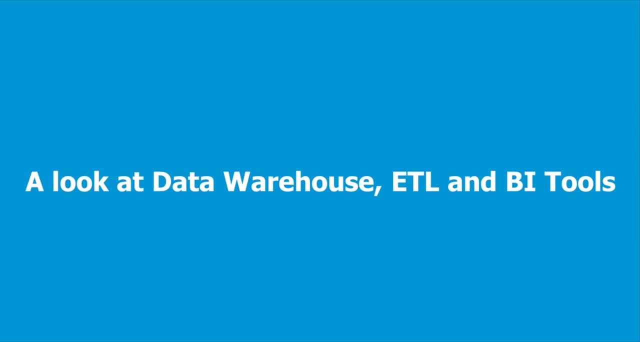 But broadly speaking, these are two separate items rate. okay, there is a question: what are the importance of bi? so, ashish, when i talk about the bi, how are the best i can explain the importance of bi is that if you want to get the sales of a particular region for last five years, if you want to get the information that 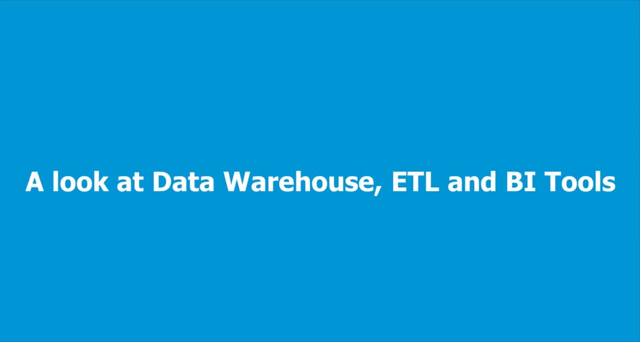 which is your best performing sales manager? which is your worst performing? which is your worst performing sales region? which product is your is great in demand? which product you have less in your store? those kind of information or those kind of questions are being answered by the bi tools or with the bi process, and this helps in taking you the strategic decision. so it is not. 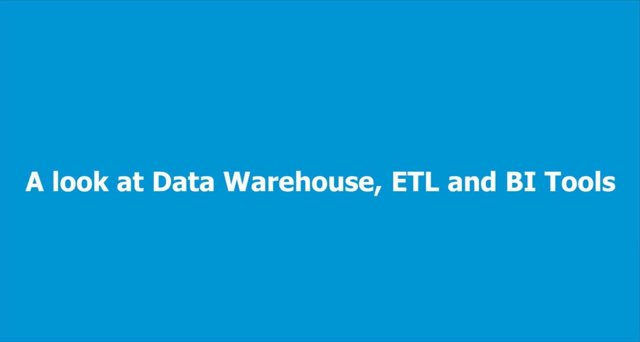 about that. you want to bring a product or you want that which product is available in your store or that is not a part of your bi right. you want to bring a product or you want that which product is available in your store or not. it is more about that which product is doing good if i am introducing this one particular product. 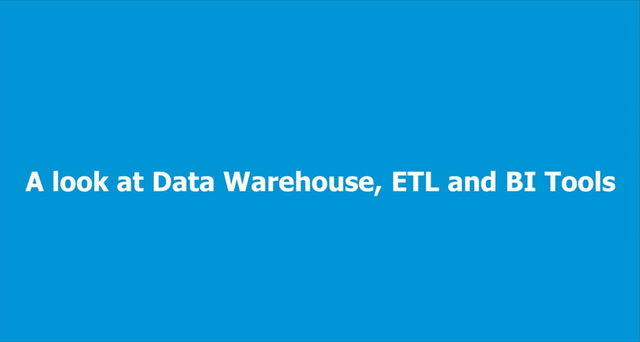 in my store. will that do good or not? there is a demand or not? okay, this particular um, this particular product will be used by children's, women, men, those kind of things, those kind of information is. those kind of questions are being answered by bi. take a look at the data. 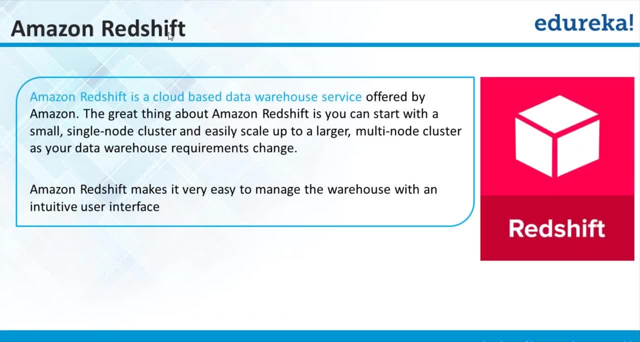 warehouse, etl and bi tools. so we have this amazon redshift, so this is something that probably winner you were looking for. that amazon redshift is one of the is one of the clouds by data clouds cloud-based data warehouse service offered by amazon. the great thing about amazon redshift is: 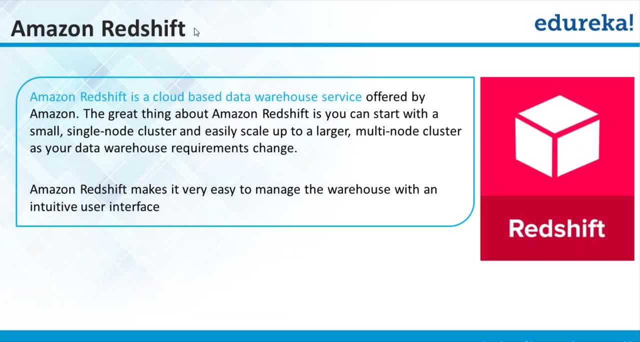 that you can start with a small single node cluster and easily scale up to the larger multi node cluster as your data warehouse requirements change. amazon redshift makes it very easy to manage the data warehouse with an intuitive user interface. okay, so amazon redshift is one of the 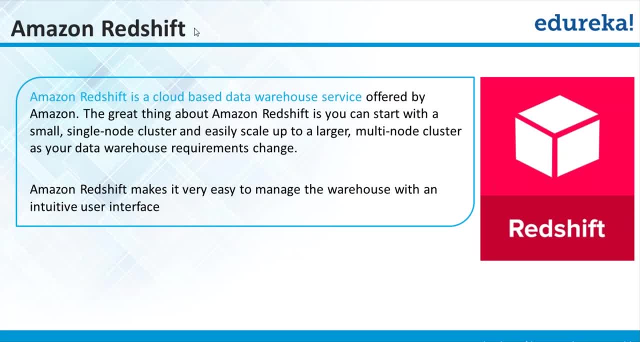 data warehouse for that uh, amazon is maintaining, uh, maintaining all the infrastructure for you. they. and again, if you go with the amazon redshift, you ask for them, they can provide you certain packages with which they can give you a bi tool. they can give you a etl tool, that how you can load. 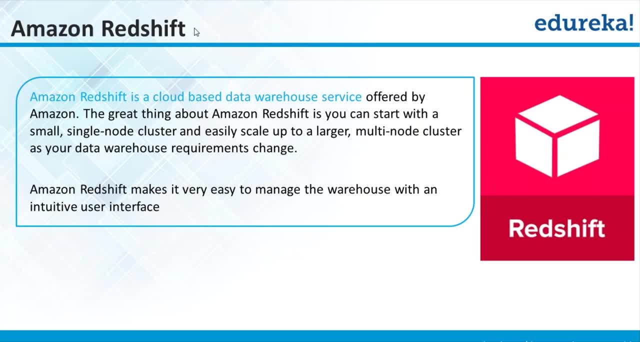 data from your traditional database into the redshift. so that will completely come as a package. okay, it is all up to you that maybe you just want to use the database of the redshift- a vision redshift data warehouse- and after that you want to do your own reporting. it could be just your plane excel. 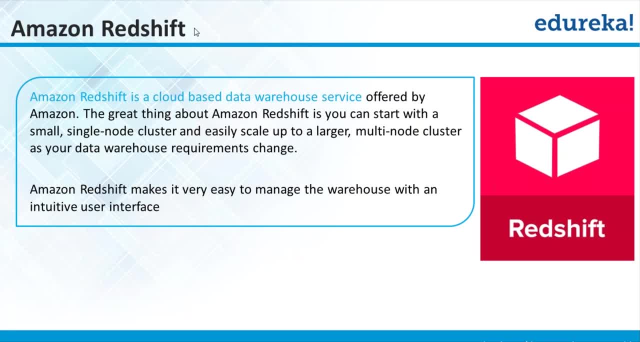 sheet, that you want to create some graph by bar chart, pivot chart, anything, or it could be a using tableau, jasper or any other tool. obi, that you want to use the data available in the redshift database- okay, apart from that, we have other tools as well, so informatica power center. this is one of the most 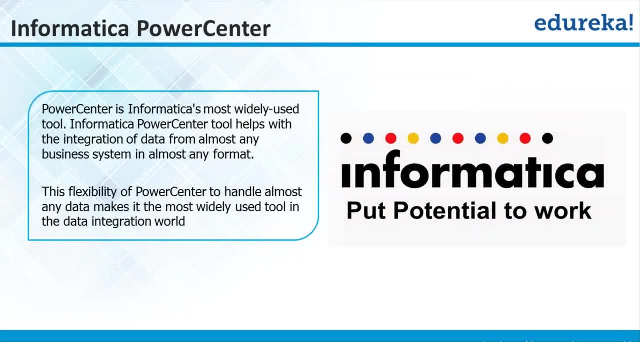 well-known tools we have at amazon: redshift大家好, informatica power center. this one of the most in the redshift database. we have other tools as well, so informatica power center- this is one of the most widely used tool which we know as Informatica. Informatica Power Center. 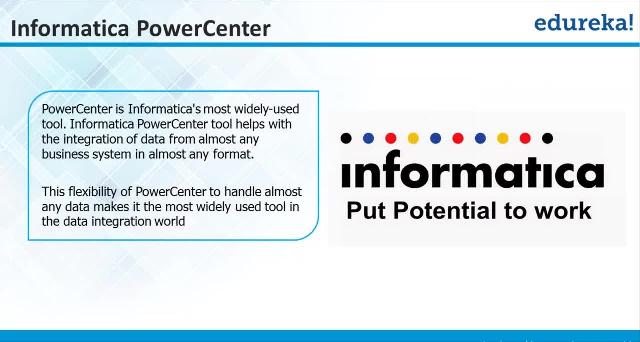 Informatica Power Center tool helps with the integration of data from almost any business system in almost any format. This flexibility of Power Center to handle almost any data makes it most widely used tool in the data integration world. So we have this common thing, common problem in today's organization that we have data. 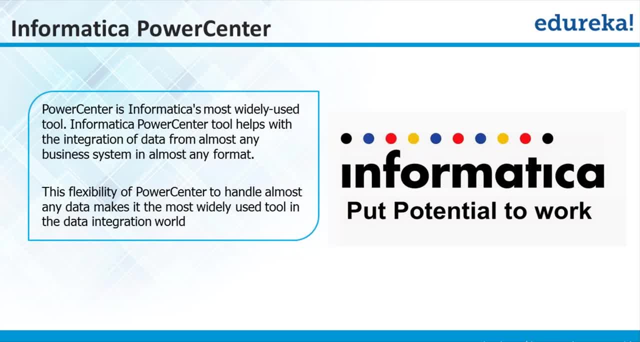 available in various systems. So at some of your department you might be having your Oracle database. Some is still on the mainframe, Some of the applications or some of the departments are still using Excel sheet And when you are talking about a data warehouse or creating a data warehouse or doing a business, 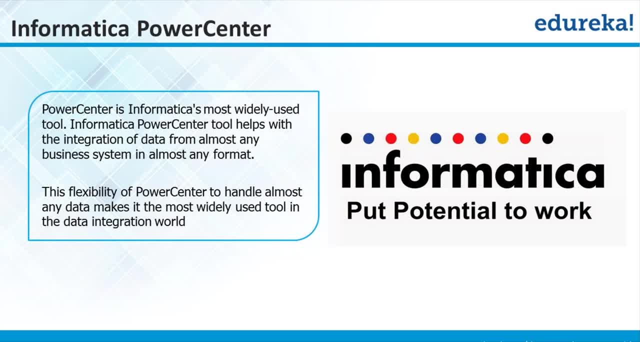 intelligence on top of that. So you want data to be, in a sense, In a single format, to be transformed in a single format. So to get data from all different format, transform that and put it into a single database. It could be anything. 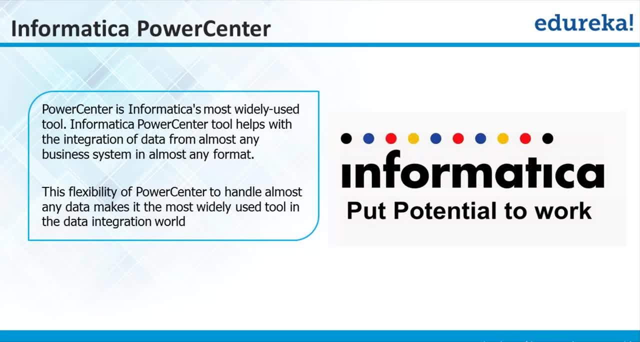 It could be a mishandler shift, It could be a green plum, It could be just a Oracle database. that is being done by the Informatica and by Informatica is very good is that it deals with almost all type of sources. You name it. Informatica provides a connector for that, not a solution for that. 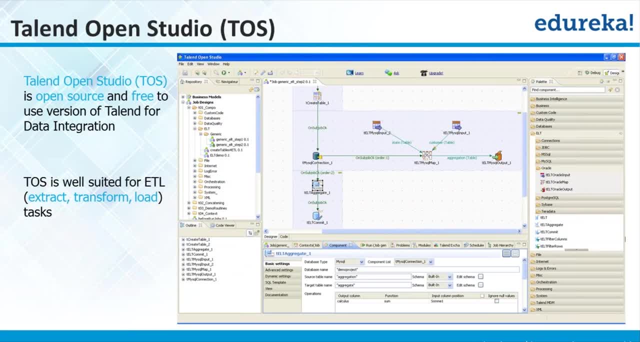 After that we have something. We have Talent Open Studio. This is again an ETL tool, but it is a free version. It is used free version of Talent for data integration. It is used for this: Talent extract, transform and load. 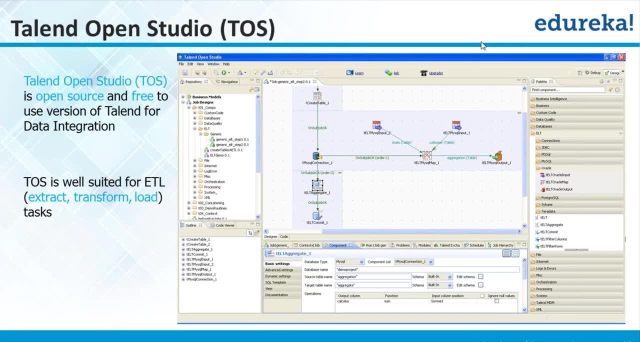 That is how you load your data into the data warehouse. So, Savitri, this is what you were asking, right? So you have your source data. You need a ETL tool. You transform that data again with the same example, What Informatica is doing. Informatica is a is a paid tool or is an enterprise tool for. 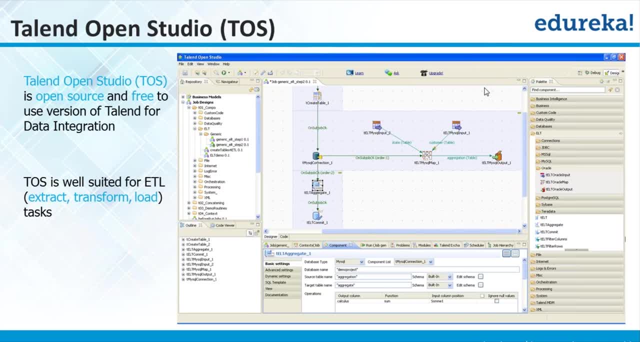 that You need to pay some cost for the licenses, whereas Talent Open Studio is a is a open source tool. You do not need to pay for the license, You can install it and you can use it for your enterprise or for your organization. 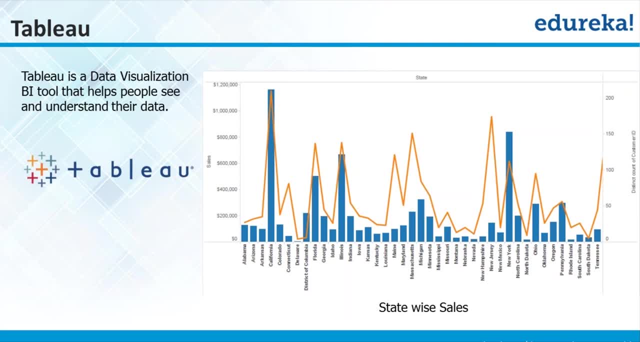 Okay, And so that was more about the data warehouse ETL tool. Now coming to the reporting tool, or what we call it as a BI tool. So you have your data available in the table into a, into a data warehouse. Now to utilize that data, you need to have certain kind of BI tool, and Tableau is one. 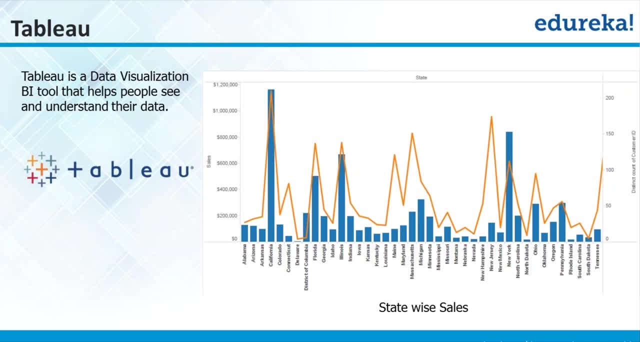 of them. Tableau is a data visualization BI tool that helps people see and understand their data, So it is again one of them, one of the leader in the markets in the BI tool it provides one of it provides best visualization available in the market. 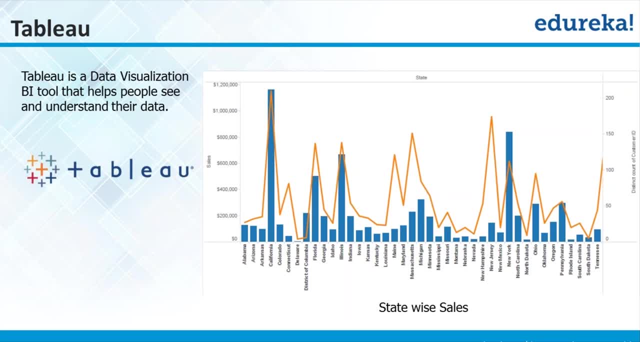 Okay. So if you have your data, you can get N number of charts. You can get N number of stories, visualization, everything from the, from the Tableau, And with the hands-on we'll see that. what kind of chart or what kind of analysis that? 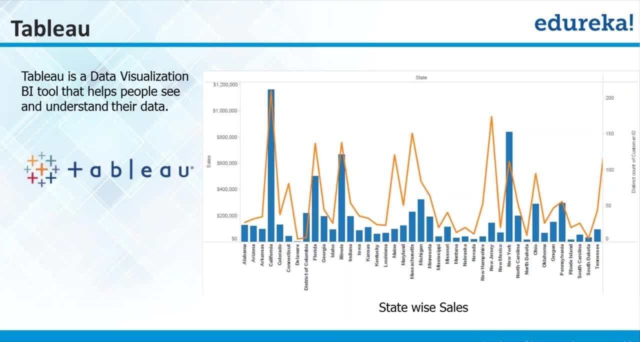 we can do with the Tableau and how, how much interactivity that we get with the Tableau. There's a question: What is the difference- advantage, disadvantage between a paid and an open source tool? Good question, Chandan So. 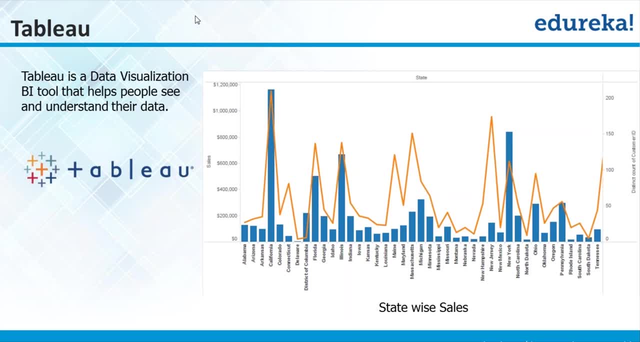 The. what I'll say is the major advantage is the is that with the paid, with the paid version, you get a lot of support with them. Okay, So you have any question, you have any problem, you get a support for that. 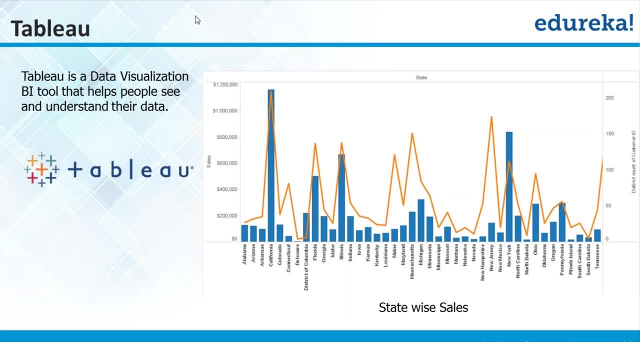 There are various features. Of course, if you are paying for something, you would be getting various features which would not be available with the open source tool. Talking specifically about the Talent Open Studio, which we would be covering as part of this module or this course, 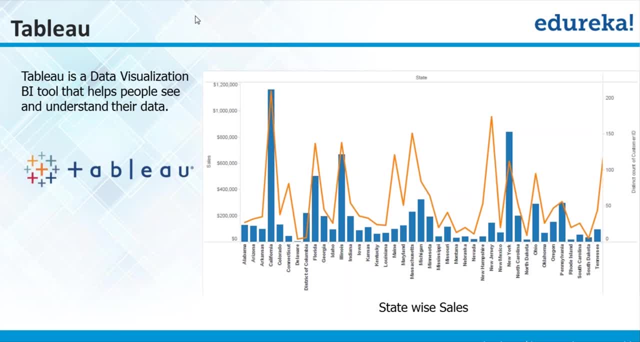 Is that. I know you've been talking about the open source version. Obviously, the talent is also available in two source, in two modes. One is that the open source version, and another is the commercial version, what we call it as the enterprise version. 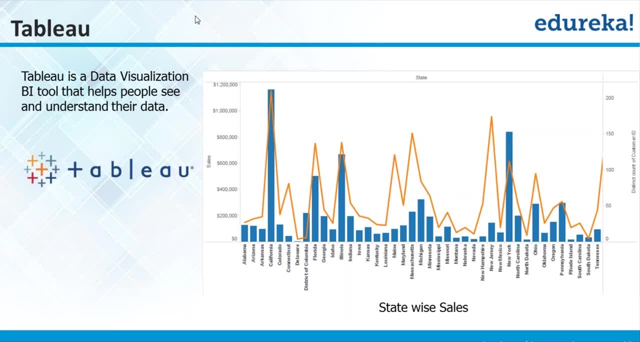 So with the open source version you can. you can do basic. you can do all ETL, I would not say basic ETL. You can do all type of ETL. You can connect to any type of source. You can write to any type of targets in any format. 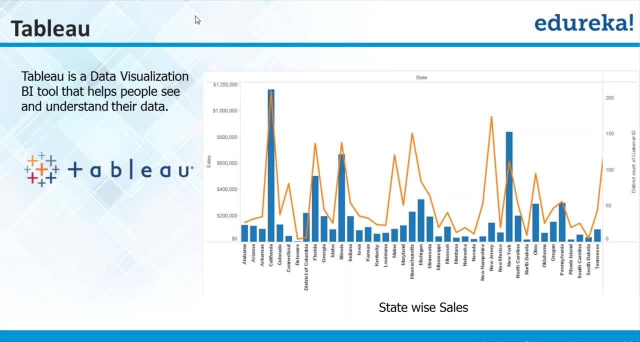 But there are certain things such as versioning, Maybe integration with the soft Subversion management that is available with the enterprise version. multi-user login is available with the enterprise version, so you can, you can install, your install the software at the server and you can have various clients connecting to that. that. 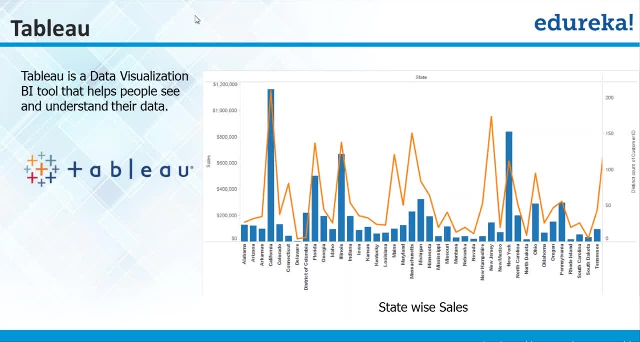 is available with the enterprise version, whereas with the open source version, you need to install it on your local PC only or at a single machine only. apart from that, you have something as a administration center with, in case of talent, that is, talent administration center, available with the enterprise. 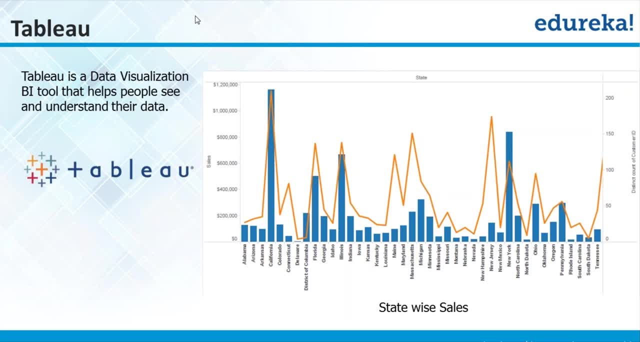 version where you have job scheduling, monitoring kind of tool, okay, whereas with the open source version you need to do it manually. though there are options available that you can export that as a export, that as a dot bat file, dot SS file, and you can schedule it via Windows scheduler or a or a unix cron. 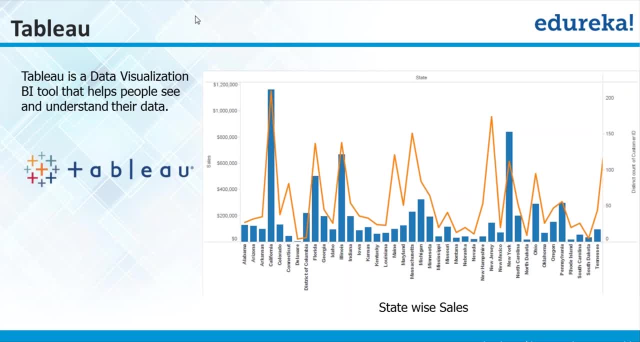 file. so all those facilities are available. but of course, if you are paying for something, then you you would be getting some more additional, additional features and again it depends upon the need of your organization. so if it is a big organization, you want to do this kind of. 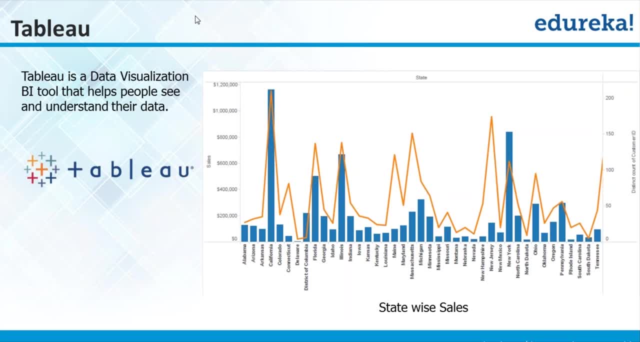 monitoring that, how your process is doing. you want to schedule it where that you have a big team, big team working on the ETL project. you want to have a certain kind of configuration management, each one logging into that, have certain kind of versioning. so for that enterprise is the best option or the commercial. 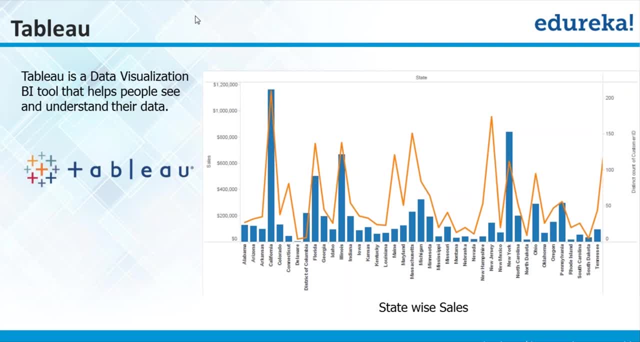 license, whereas if you can manage with the with the open source, and the best part is that it is open source- and you can manage with the open source, and the best part is that it is open source and the best part is that it is all java-based, so it is a free version, you have your infrastructure available. 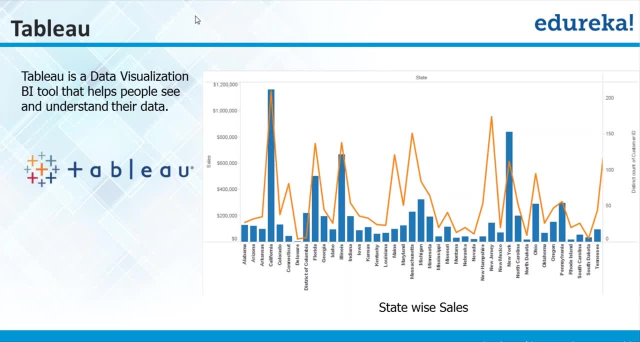 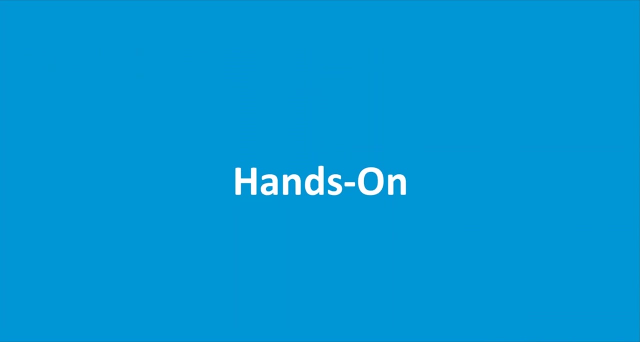 you just install the software and work with it. I hope that answers. is it open source tool tableau? no, sorry, three tabloids. tabloids, not open source tool. tableau is a paid tool. we do not have a open source or a community word version of tableau, so I'll get into the hands-on that. I'll show that. 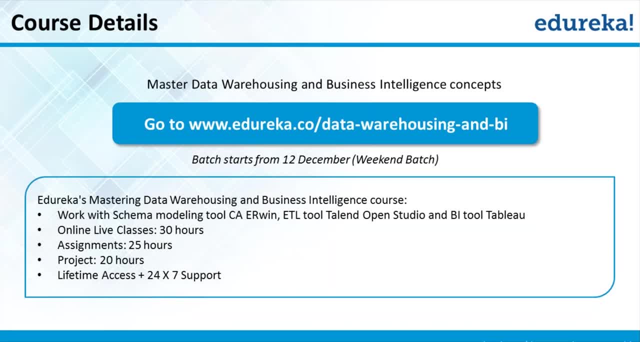 what are ETL things that we can do with the talent, or what kind of report that you can do with the, with the tableau, uh, whereas these are- these are the details about this- uh course. data warehousing and business intelligence. we have this badge starting next weekend, that is, from the 12th. 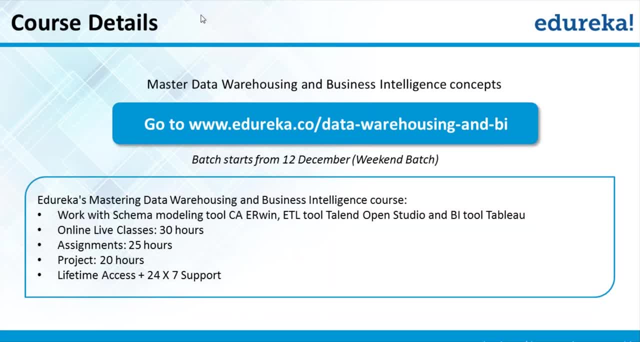 of december- and here are the details. you can check this on the website as well- that we have this. we would be covering this: data modeling concept, data warehousing concepts and business intelligence concepts, data modeling hands-on with ci, urban tool, etl with talent, open studio and reporting. 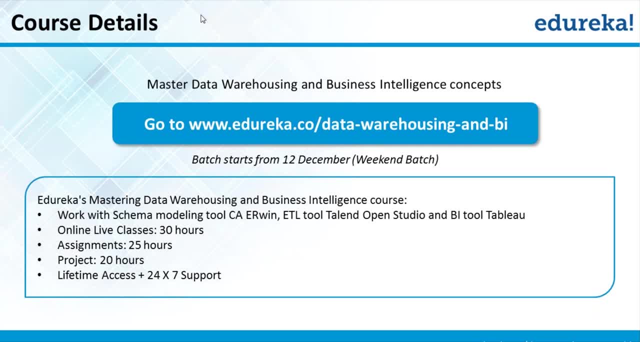 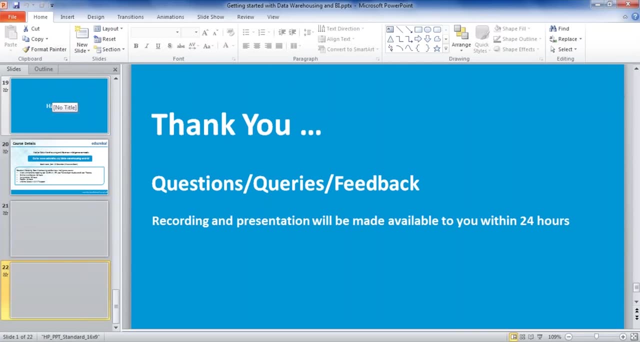 or a bi analysis using the tableau tool. it is more of a hands-on exercises. you can get these details. i'll move forward after this. so we are done with this. after your webinar is done, probably you should provide your feedback. that will help us to improve the quality of. 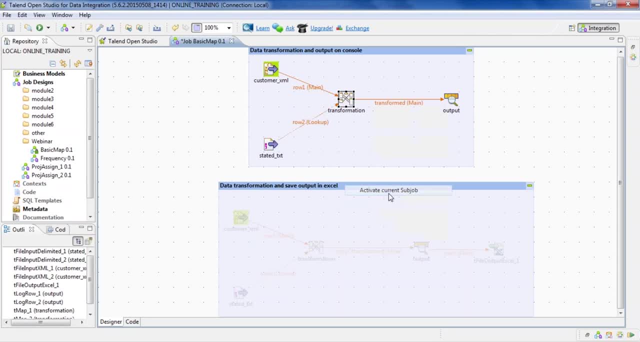 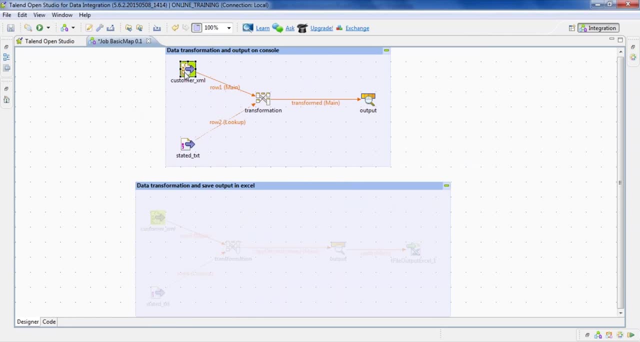 the sessions. okay, so, um, coming into this, uh, i had this simple transformation job. where you have something available in the uh, where you have something available in the xml file, something available in the text file, then you transform that data and store it into a single file in the. 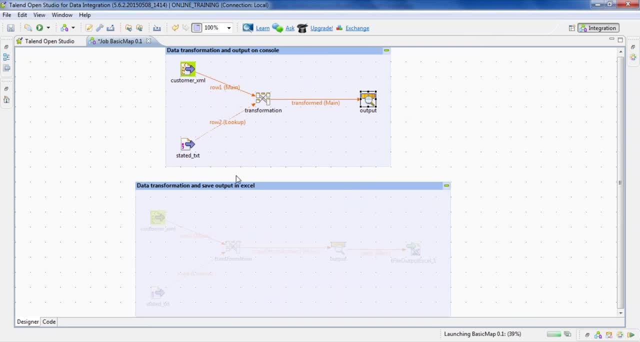 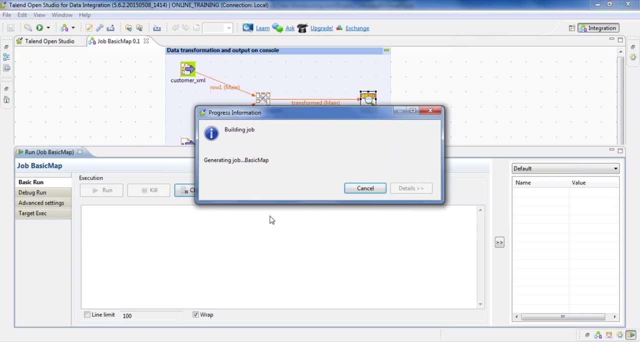 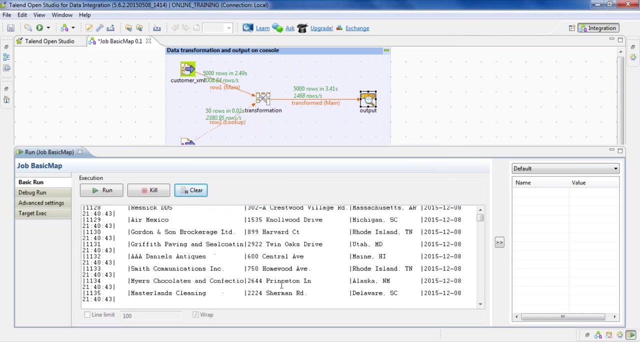 in this case, i'm just storing it into a or i'm just displaying it onto the console. that how you're getting your data. similarly, i can store that into a database, i can store that into a excel file, into xml file, anywhere. and how this works with the talent i'll show you the file. 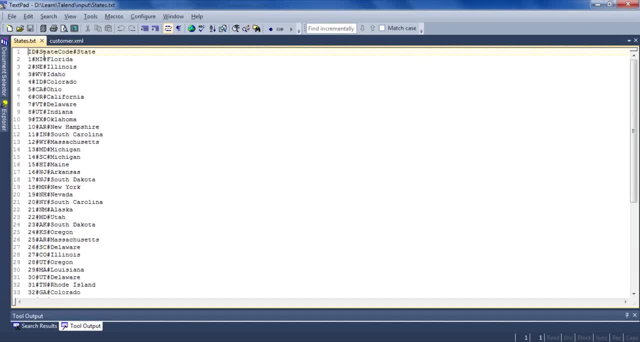 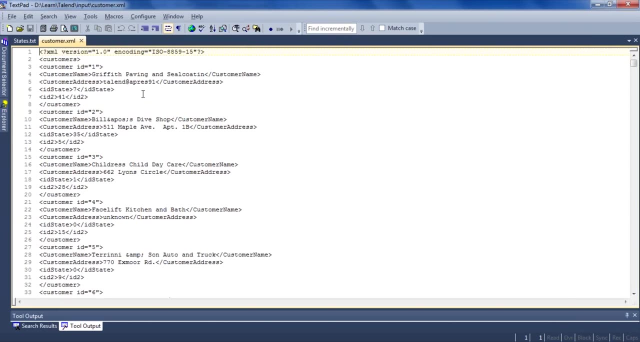 in this. i had something, as i state, on dot txt, that is, a dot txt file in which i had data which is hash delimited. okay, i had another data which is available in the xml file and probably those of you have worked with the xml you would know that how difficult it becomes to work with the xml. 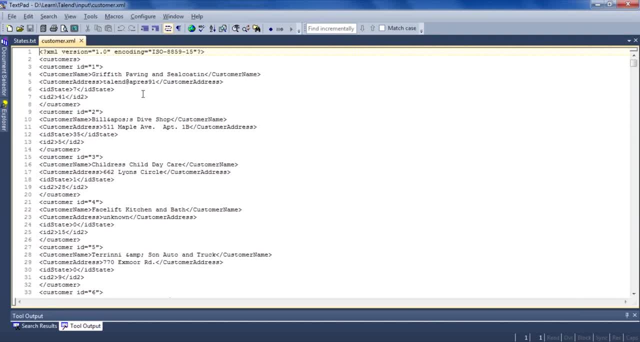 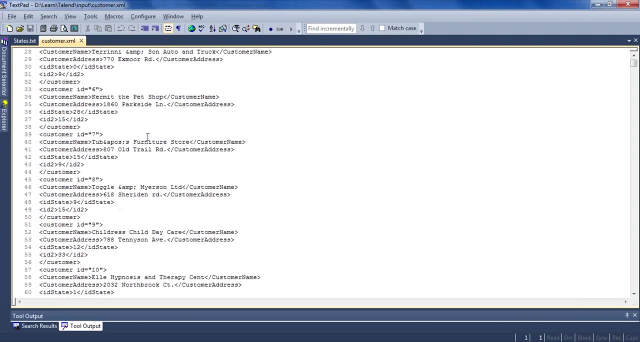 mostly in case of loading data from xml to the database or from my xml to the excel sheet. it is very difficult, but with talent it is. this whole job would not take more than 15 minutes into, or five to ten minutes, okay, once you know all the concepts. so that is how easy it becomes. so 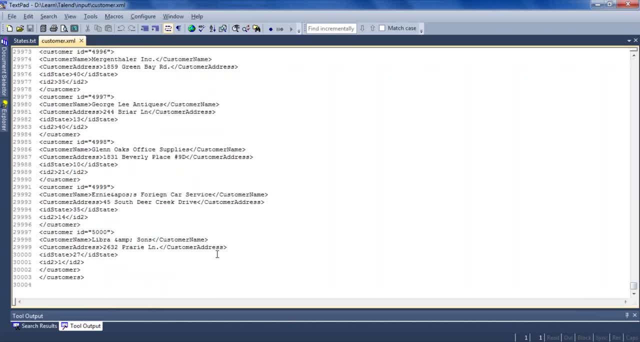 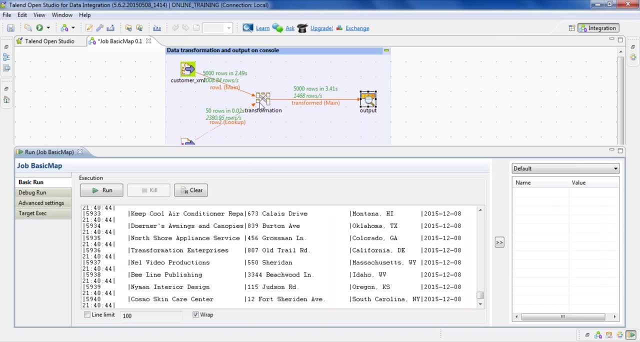 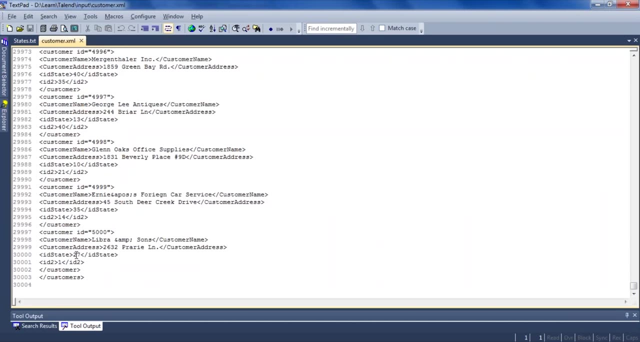 here. you can say that it is a huge file of approximately 30 000 lines and we are loading that in a matter of seconds. okay, and what we are doing is that, if you see this customerxml, we have something as a customer id name address and in that we have something as a state and that state. 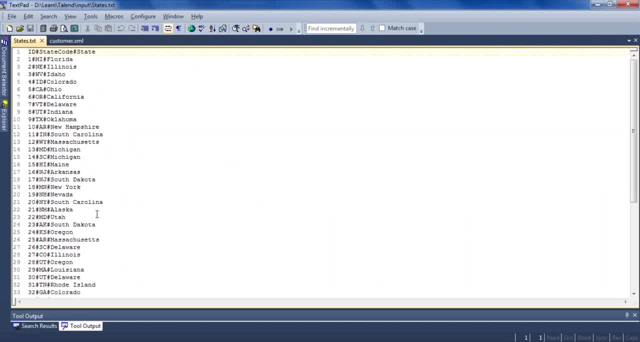 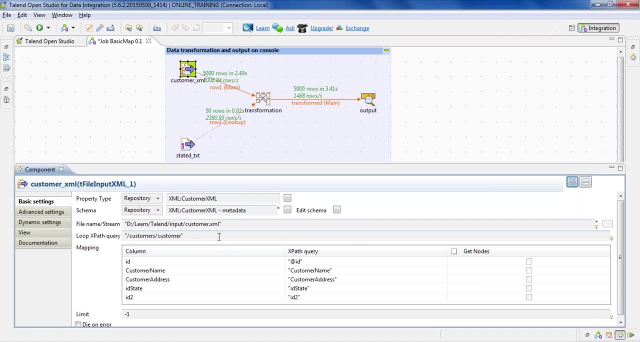 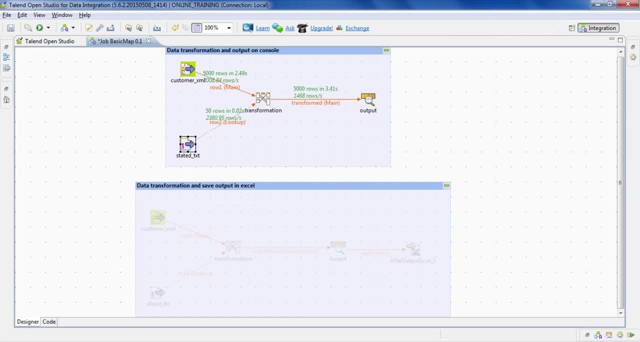 is looked up using this state table. okay, so how it is working is that i can use some. i can configure all this, all this component, that how to read the excel file, i can. similarly, i can configure how to read a text file, and then i can configure the file, and then i can configure the file, and then i can. 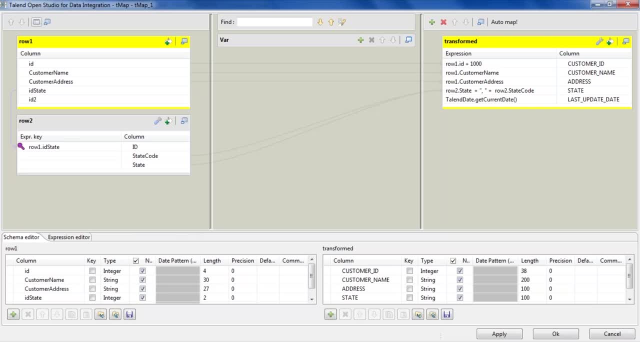 do a transformation based on that. so there's a tmap which is available with the, with the talent tool. there you can join the uh, join on the column. you can do a transformation over here that you want to append something, you want to add something, you want to get the current date. that is what is. 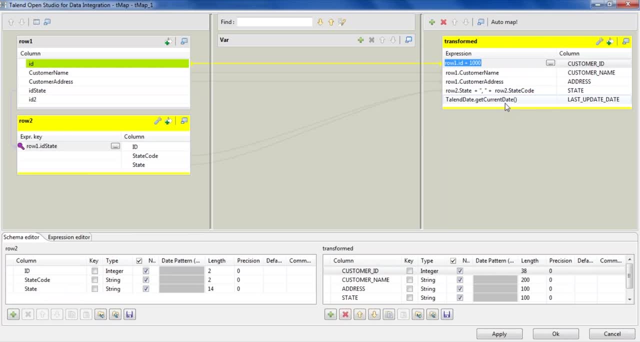 required with the, with most of the atl tool, that when you loaded your data, when you last updated your data, there are various types of joins available, that it could be a left auto join, it could be a uh inner join or a left out join. it could be a left out join or it could be a left out join. 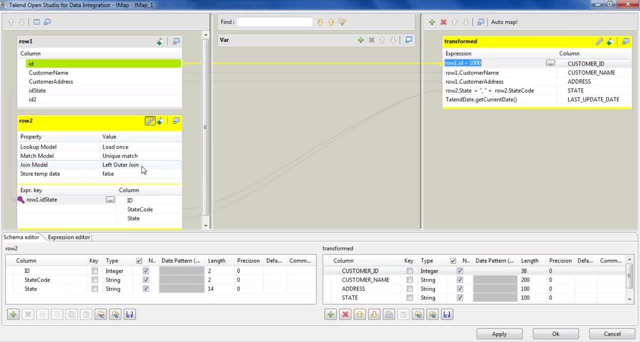 it could be a left out join. how you want to use your uh, how, how you want to use your lookup, that load only once. load every time. load one with each and every record so that all thing that you can do with that, all thing you can do with the talent- and again this is one of the very basic- 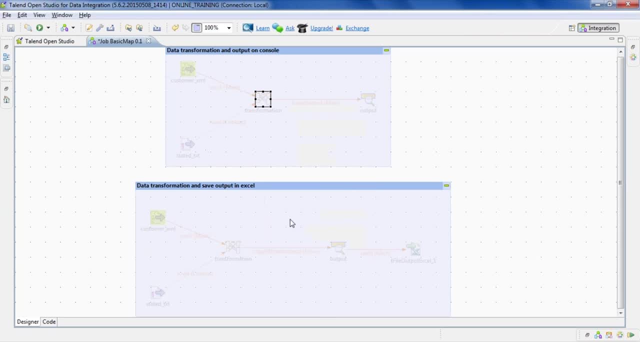 basic job, similarly- uh, it is the same job, but only thing is that i am ensuring that you should Spring-Get your content, for example on Notepad service, and how we can easily take the slice that will take your title back your folder and create your file. you can see. 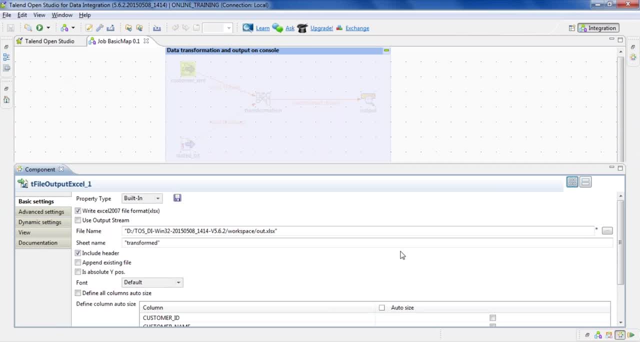 that by by by ش. NCAA needs a file when you're building your content and somebody has the 10 client champ so you don't have to bother try these simple things later in that field. so you just done a little stuff and now it's been created by the Arenal final. we're going. 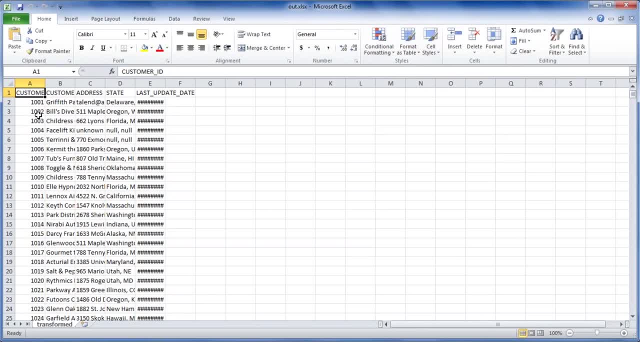 to transition andеру, so the sechs packages. uh, and then i am07y really open. what i mean is we would do two jobs are so, which will be based on this table called subject model. we actually have a one sentence function you can do. you mean you actually use such data in the next 앨. 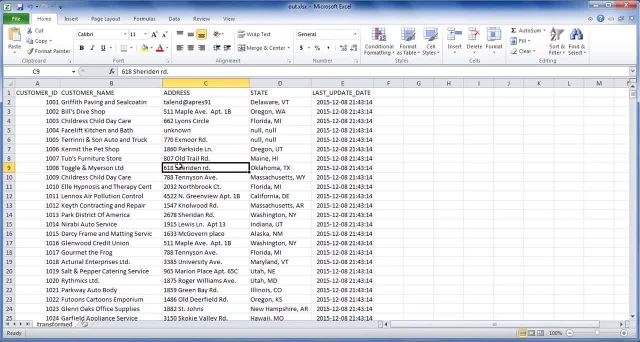 file withinящrezing authority and you might be asked to communicate a conflict function to thenehmer file, and lately we stored that. after transformation that we, we concatenated state, we added something. we added some value to the customer ID. we can generate our own customer ID as well. we appended the customer names and then we generated. 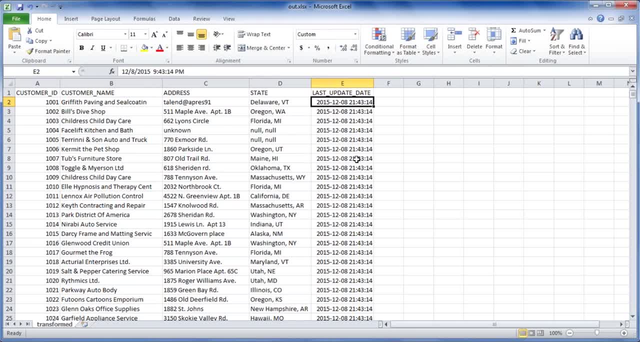 that last time when we updated this record or when this data was created, all these things, and if you can see that it is, it is around 5,000 records. okay, and this is how you can load it into a. we have this header as well. this is how you. 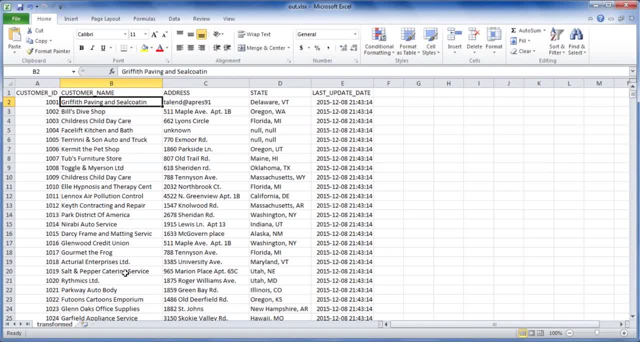 can load it into a excel file. similarly, you want to load it into a JSON file. you want to load it into any of the database. it could be anything. it could be your msxs, mysql, oracle, postgre, redshift or anything. talent provides connectivity for that or connectors for that, and there are certain questions. developer. 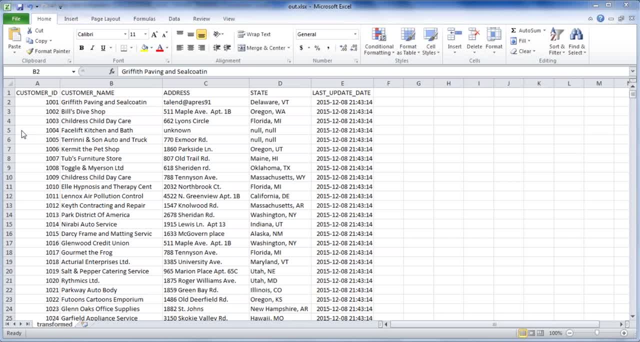 experiences count if I develop a experience and if I don't have a developer experience, and if I don't have a experience as count if I switch into the BI. yes, definitely so. if you have some development experience, then these things- that how to transform your data and all- 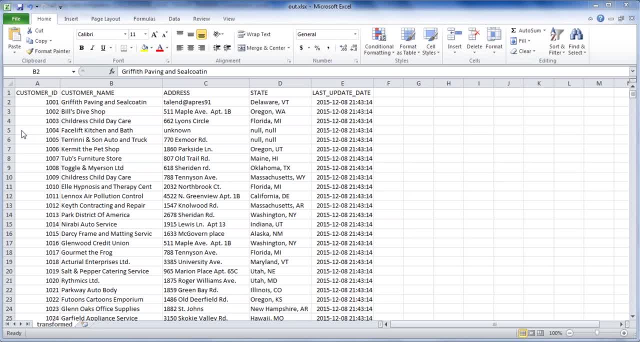 these things becomes very easy when you are moving into the BI area, that you know your data, you know the technical details about it. there is another question: give us some information on how tableau is different from Informatica. why is it necessary to use tableau? so, talking about 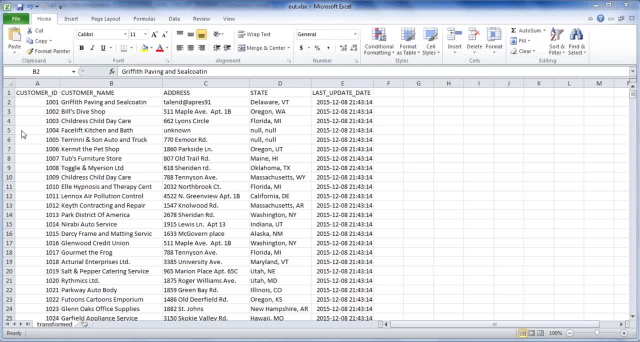 this. what's? what's the difference between the tableau and Informatica is these two are different products altogether. Informatica is all about the ETL, that is, extract, transform and load, so maybe we can compare Informatica with talent, whereas tableau is entirely a different tool which is used for 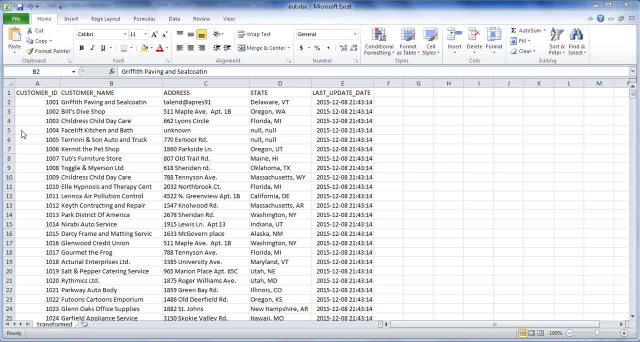 reporting, for generating the, generating the report, generating the visualization using the data which is stored in your database or your data warehouse, and now comparing between the Informatica in the, between the Informatica and the talent. is that yes, Informatica is the is a leader in the market right now, but 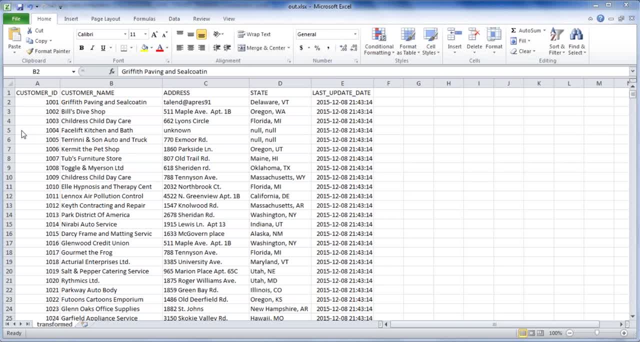 problem with the Informatica is that it is a licensed software. okay, so that is bit of costly, of course. performance wise, you get a good performance with Informatica. you get good connectors with Informatica, but similarly you get all those connectors and everything with the talent as well. talent is, talent is. 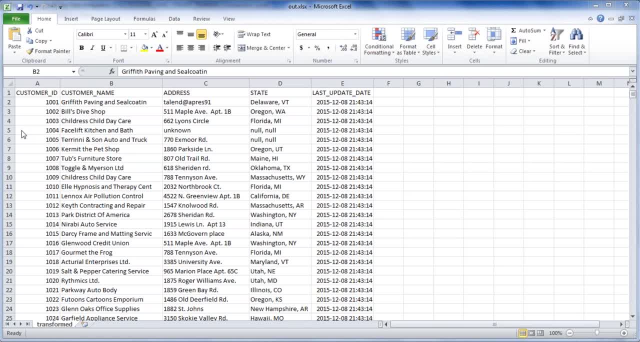 comparatively new in the market and it is a little bit more expensive than the- and sorry, i almost getting question. so talent is comparatively new, as talent is game comparison with you in the market, but it has picked the very well because of the, because of its open source architecture. 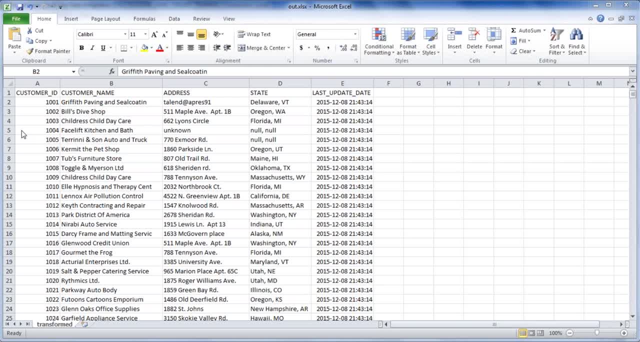 right. so that is the main difference, and even if i talk about the commercial edition of talent, the license cost is comparatively less than the Informatica licensee cost. So these are the couple of differences that I can highlight right now. Let me know if you need. 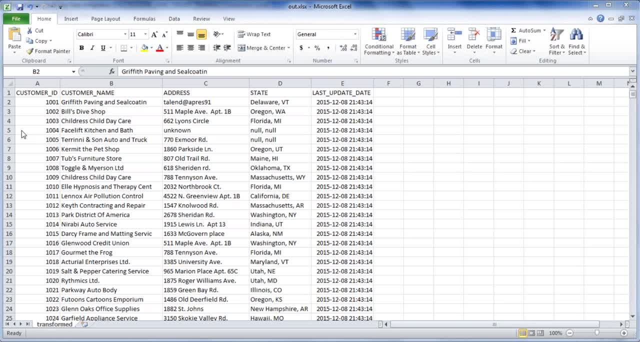 if you're looking for something more specific, Is there any open source tool available similar to Tableau? Yes, there are couple of open source tool available with the couple of open source tool available in the market. but when I talk about the visualization, 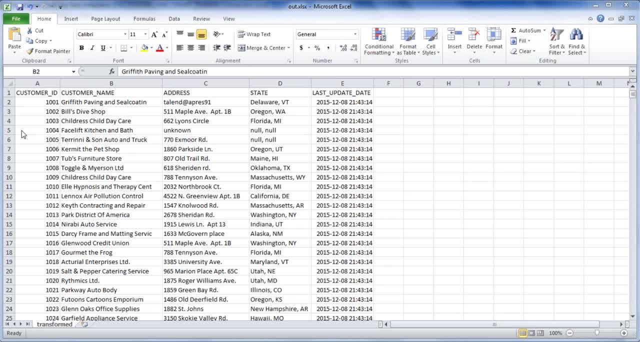 Talent provides the best visualization, so there is no comparison for that, and that's the reason we have Tableau, even though it is a licensed software. Okay, apart from that, there are something else that you can do: some UI work. you can do some visualization. 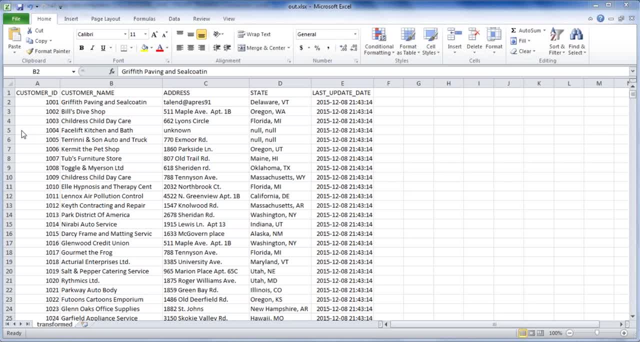 using the programming languages. Okay, so you can use jQuery, you can use D3 libraries that can hook up with your JavaScript and all, and that way you can build a visualization or you can do a BI using the JQuery. So that's the reason why I'm talking about. 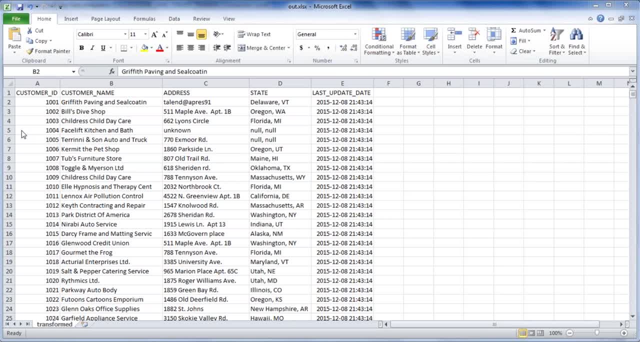 freeware tools, but if I talk more about the tool side, then I don't think so there is any freeware competitor for Tableau as far as I know. There's another question. please show us the data to be loaded into. 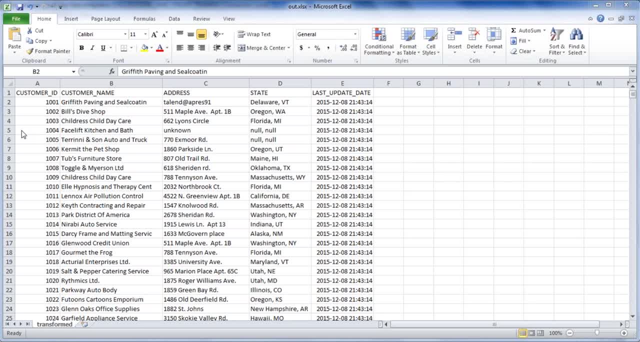 to be loaded to the data warehouse. So when I say that I need to load some data, so this is more of a sample data and I think this find for the because if I'm going to take a big data or take a huge amount of data, 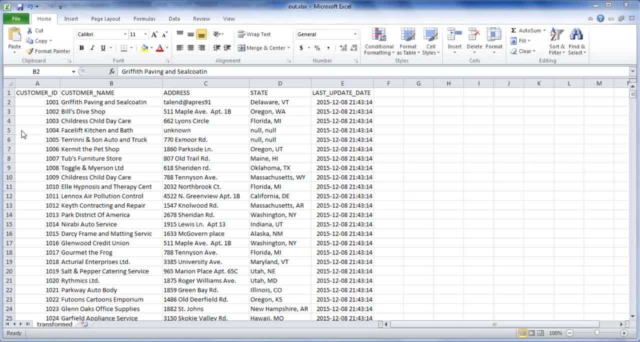 it will take more time and we'll go out of time for this webinar. Okay, so this is the sample data and this is how you'll get this data. So here I'm, having only five tags, or 10 tags in my customer file. 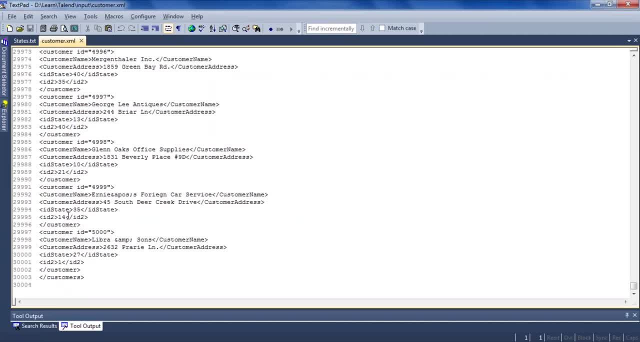 It could be 20 different tags. I would be getting something as a product, product sales and all those things. So that thing or that information from your database. it could be either in your Excel, Excel file, XML file. it could be either in your. 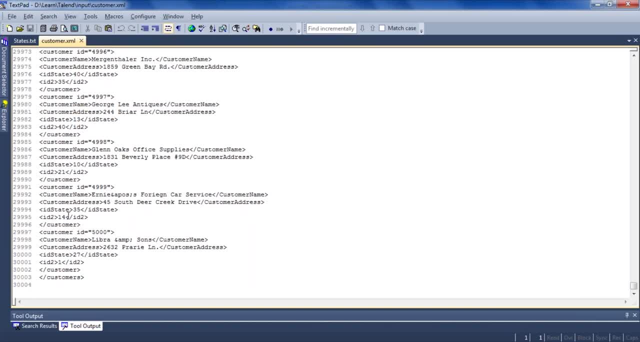 some of your RDBMS database. You take that file, you transform that data. you have some of your reference data or lookup data available in any other format. You can join that and if you see that we can join with the different different sources. 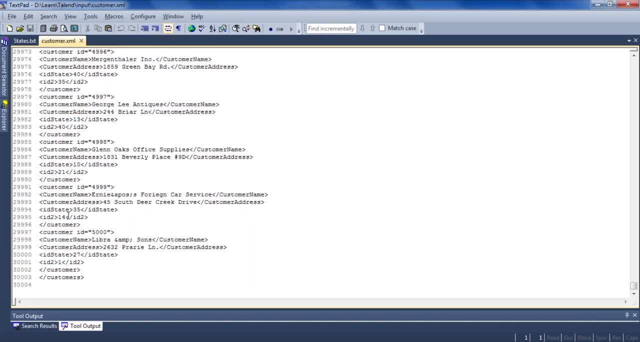 So if I say that you have some data available in XML, you have some data available in text file and you have some data available in your RDBMS, load that data into my data warehouse. That will take too much of time for you. 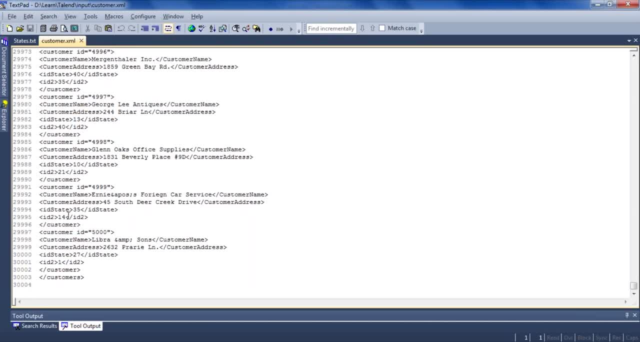 because you need to write a huge line of codes for that, Whereas it is very simple with the Talend, or with any of the ETL tool for that matter. I hope that is somehow that answers your question. due to the limitation of time, 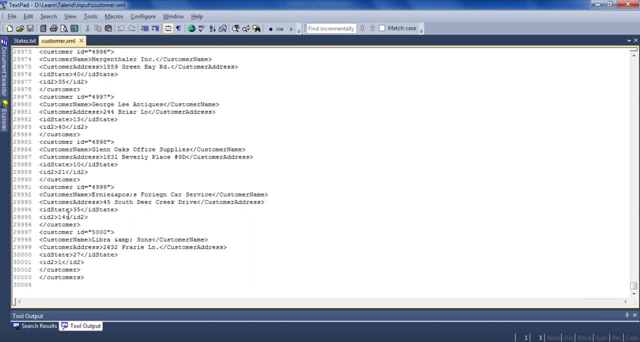 There's another question: where do the tools like Talend fit with the? Talend fit with the Hadoop. So Talend provides very good connectivity with the Hadoop or with the big data components, If I talk about the Hadoop or the big data. 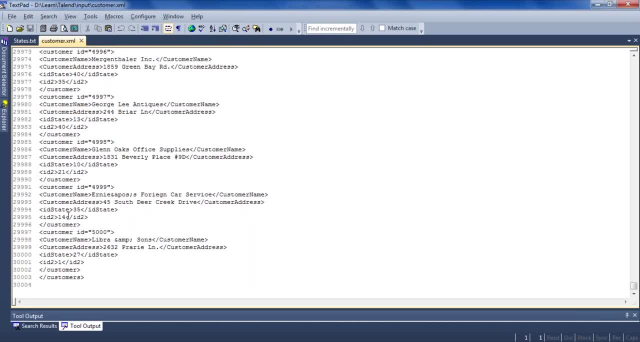 for that you need to understand the map reduce programming, peg, hive, those kind of things, Whereas with the Talend you don't need to go into that, You don't need to understand, or you don't need to learn the Java programming as such or map reduce programming. 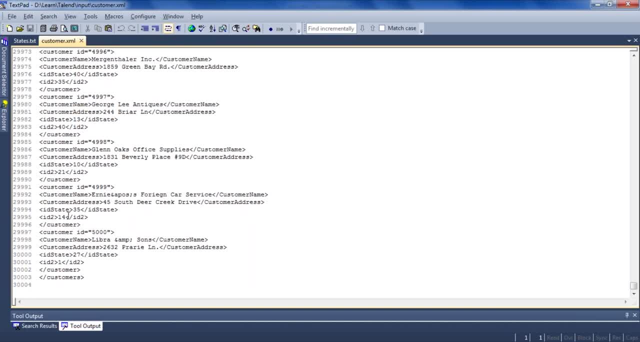 Because Talend, being the ETL tool, does work for you at the back end. Okay, you just need to configure the tools, you just need to make the connections, you just need to write the logic. Write the logic as in using the using this components. 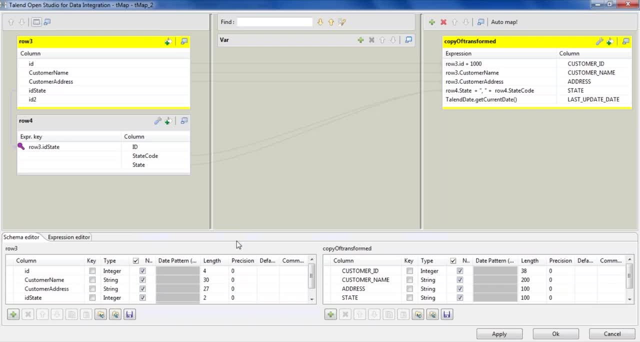 that? what all transformation that you want to do, Like we did in this, the map component, and after that Talend will write map reduce program for you at the back end, or a peg is working for you in the back end, So it integrates very well with the big data. 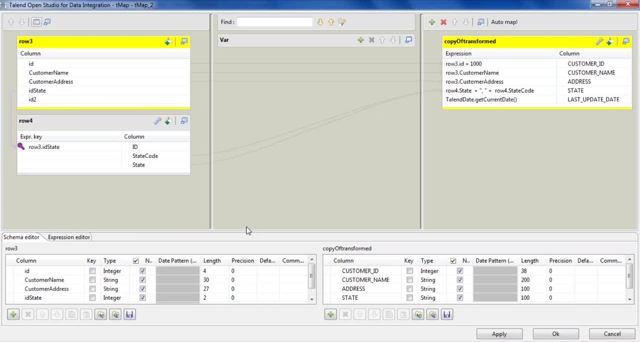 with the Hadoop. What are the major? going to the next question: what are the major skill knowledge required for BI? Please tell us career in BI and eligibility criteria in every organization need BI. Yes, so Ashish. every organization need BI. 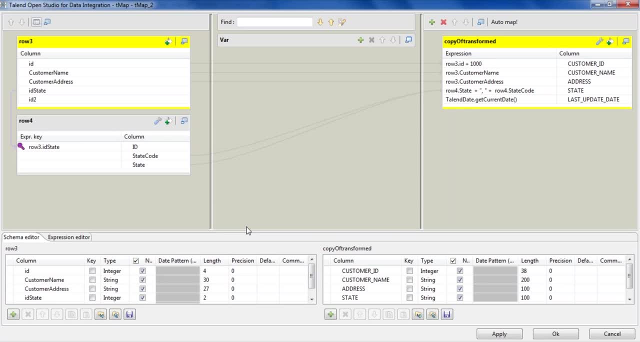 That is very true. You can get into the BI, or with the BI, or with the data warehouse. there are a couple of options. You can get into this ETL developer role. you can get into this BI analyst role, BI developer role. after that you have further path. 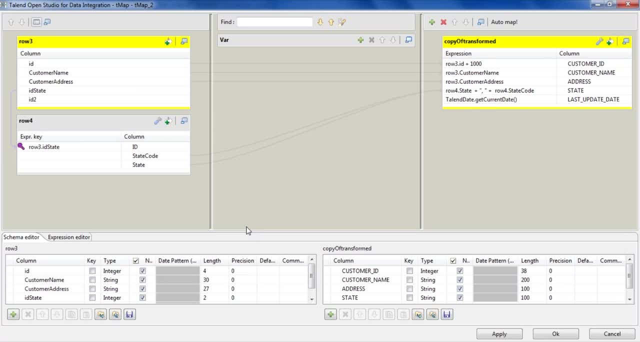 of a data architect, data mining, data scientist, because once you get into the data, there are a lot of openings And you might be knowing it very well that all the talks or all the positions that we are having in the market right now is more related. 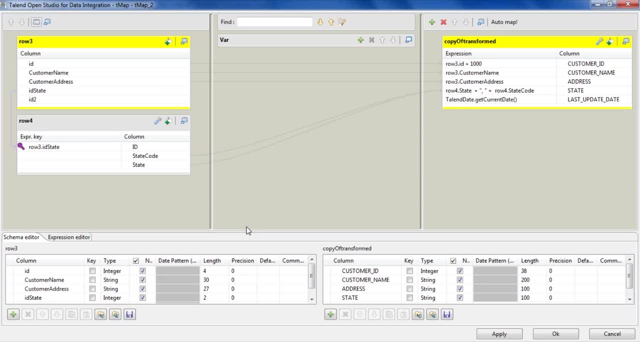 to data. It could be your data analyst, it could be a database developer, it could be a ETL developer, data scientist. So once you know your data well, you're good in the market. And this data warehouse, business intelligence, or this concepts ETL data warehouse. 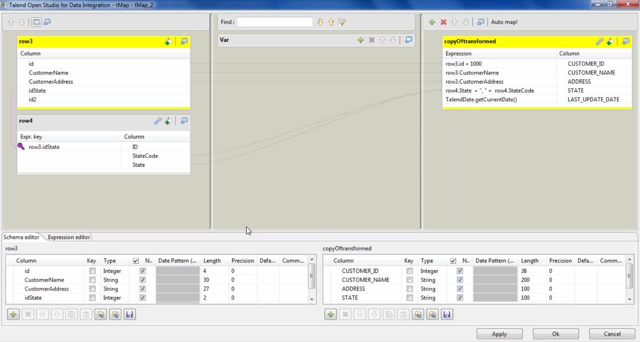 all these provide you platform for that. I hope that somewhat answers your question. Please share your questions towards the step-in talent for the ETL. Okay, so when I say that ETL, ETL could be a very- it could be a very big thing that you are getting data. 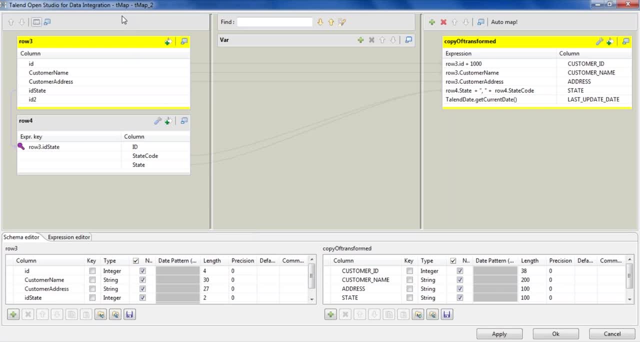 from different, different sources. You are doing a transformation, that you are doing certain calculation, you are doing certain mapping, lookup, Whereas it could be as simple that you have different sources and you are just loading data into one thing. So this, the TMAP which is open on my screen: 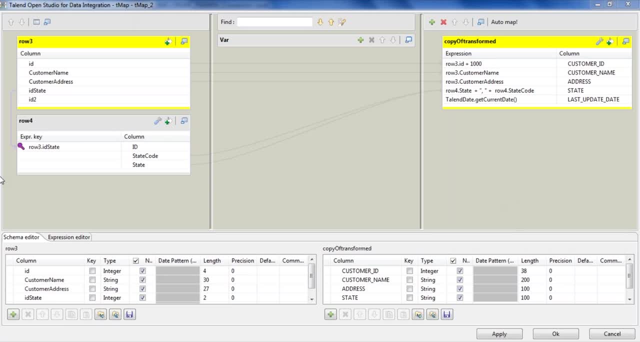 the talent is one of the example for the is one of the example for the ETL process, that how you are transforming your. So more detailed classification of this is that I have something. these are my extracts, these are my raw data. 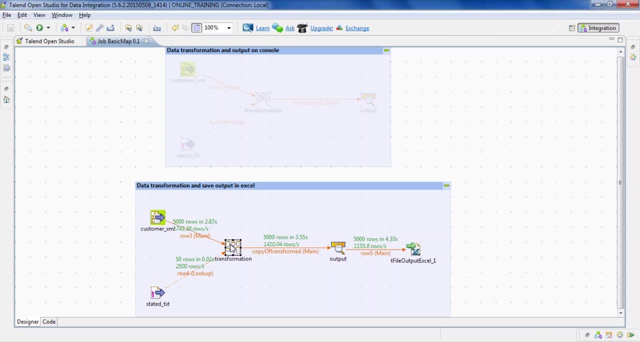 I am transforming my data using this transformation. Transformation it could be just mapping of some data, doing a lookup on those kind of things, And after that I am loading my data into my output file. It could be a Excel file, it could be a data warehouse. 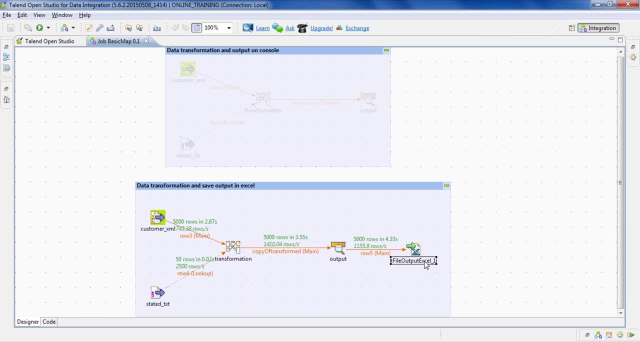 anything. So, in simple terms, this is all about ETL, what we are doing with the talent. There's another question: how will you differentiate data warehousing and BI with Big Data Hadoop? Can you brief on the same? Yes, Vinay. 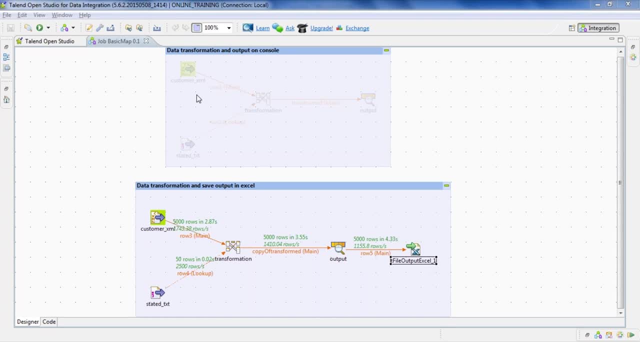 Vinay, I'll quickly go into this because we are- we are nearing the completion. So when I talk about the data warehousing and business intelligence, data warehousing is more about the relational data, okay, And we are doing BI on top of that. 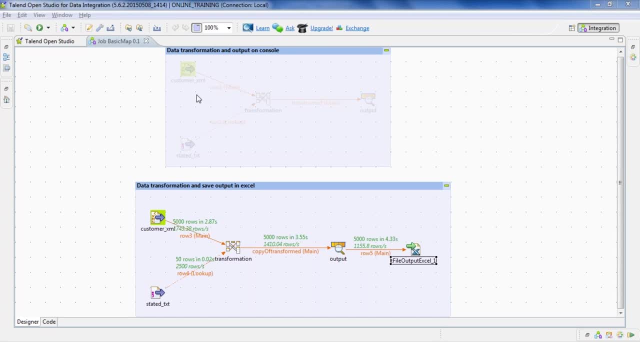 Whereas Big Data is storing a huge amount of data. It starts with several TBs, two petabytes and so on. Okay, and on top of that, Big Data again. when we talk about data, there has to be some analysis on top of that. 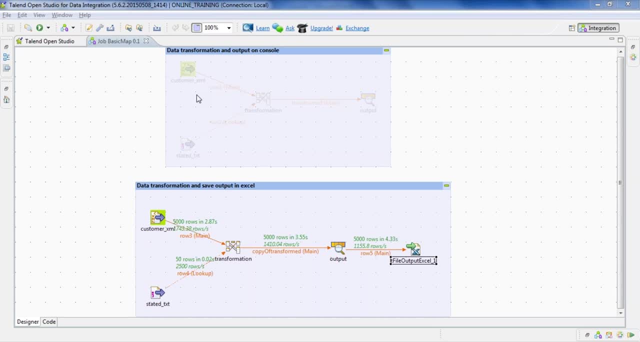 Then only your data will make sense, So we can do BI on top of your Big Data as well. Okay, it has to be presented in a way that you can take some business decision, you can make some strategic decision out of that data. 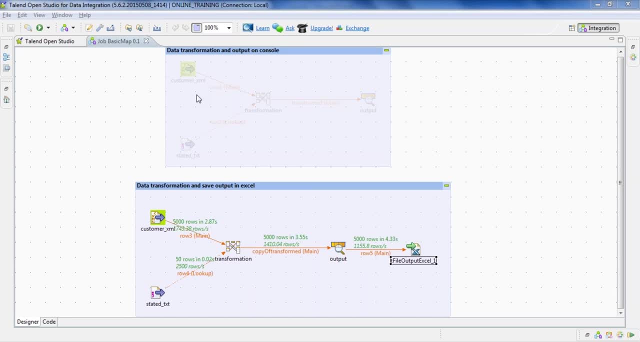 That is how BI data, or ETL or Big Data, will integrate itself. Ashish developer experience is count if I switch to BI. Developer experience is yes, Ashish developer experience will count if you switch into the BI, Because when you are switching into the BI, 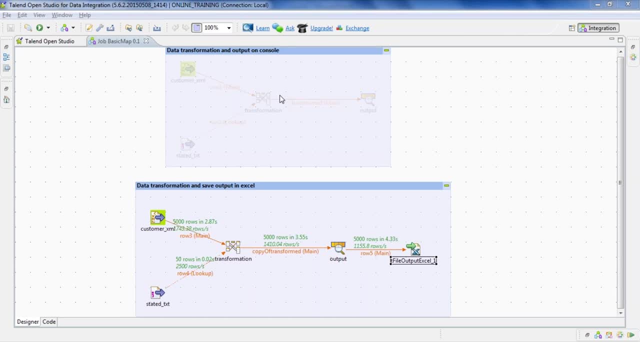 your domain experience will count. your developer experience as in your database experience, your knowledge- all those things will count. So yes, Definitely being a developer. that will help. How easy or difficult is learning Informatica for a manual tester? Are there any prerequisites? 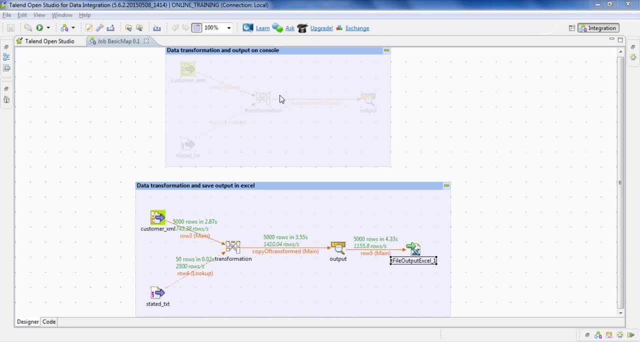 Yes, there are certain prerequisites, that you should have certain knowledge of the databases, data warehouse or business. So when I say that you need to learn a tool, tool is just doing a work for you, But before that you need to have your concept set. 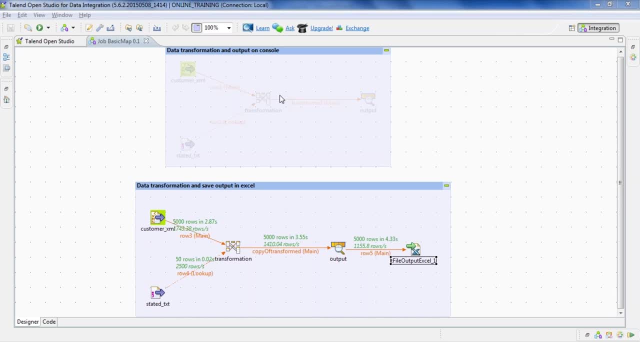 That, what is data warehouse, How your data should be stored into your data warehouse. When I'm talking about the transformation, what kind of transformation are needed And that is what will be covered as part of this: data warehousing and BI concepts. 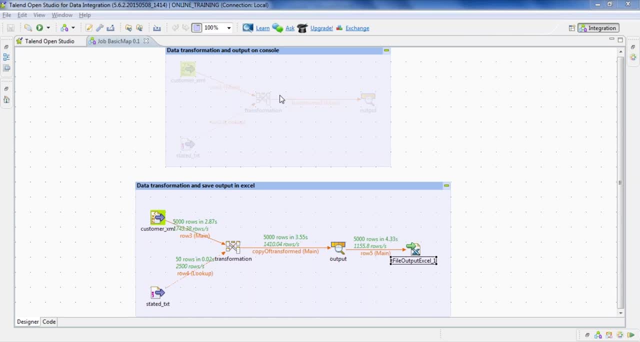 And what structure or in what format we want to store data into a data warehouse, How you can make a meaningful data out of that, And once that is done, you have your basic concepts. then you can easily move into any of the tools. 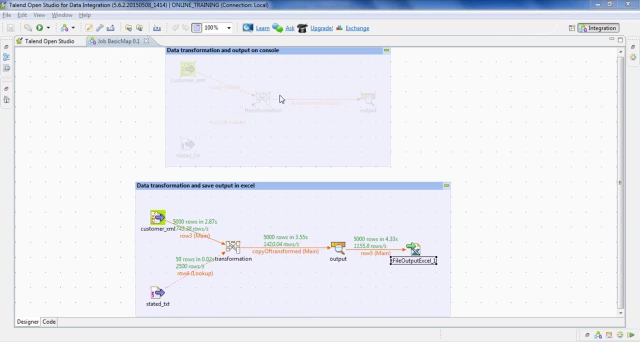 May it be Informatica, May it be Talent Or may it be any other ETL tool. Another question: difference between Tableau and Hadoop. Again, this is entirely different thing. Tableau is a BI tool, whereas Hadoop is a big data platform. 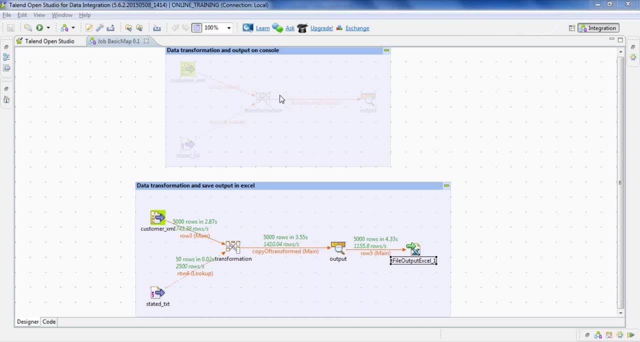 So Hadoop is again a kind- I'm not sure if I say it correctly- as a database, but it is something as that where you are storing huge amount of data, or where you are keeping huge amount of data, Whereas Tableau is just about showing data. 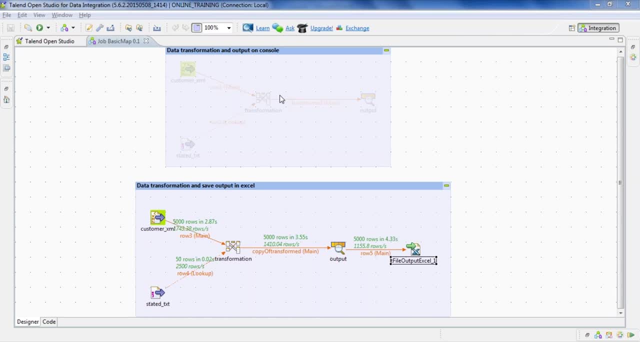 from that database. So it is like you have some data available in your Hadoop data, in your Hadoop file system- May it be, may it be Cloudera, may it be Hortonworks- And using that data available into your data platform. 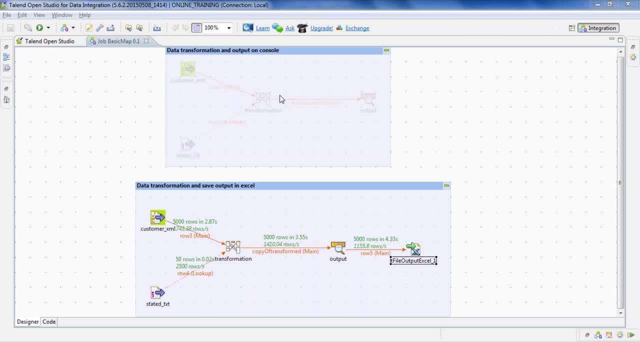 you can connect with Tableau and Tableau can generate output for you, or maybe report or maybe a visualization, for you to do analysis on top of that data. I hope that answers your question. BI is same as BO, So BI is business intelligence, whereas, if I understood, 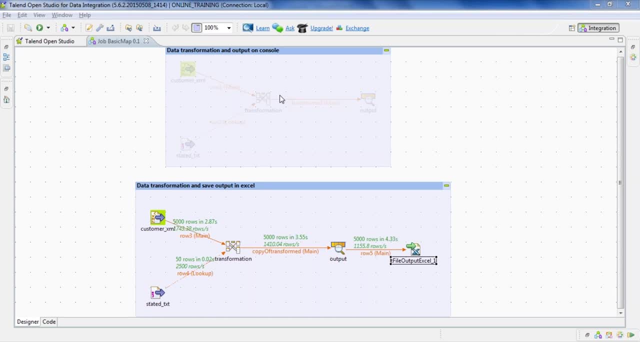 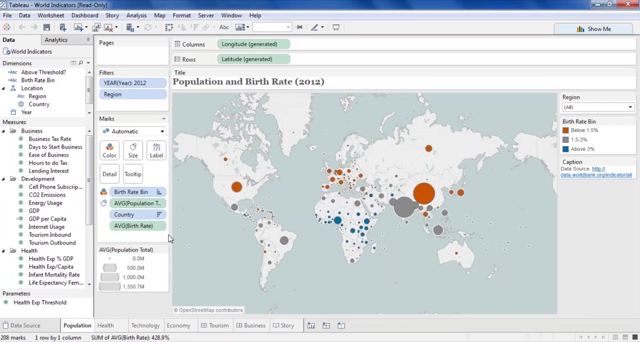 correctly, the BO which you are referring is business objects, so business objects is one of the BI tool. That is it. So BO is a business intelligence tool, if I understood that correctly, or the BO which you are referring right now. Quickly going to the Tableau part, that, what all things? 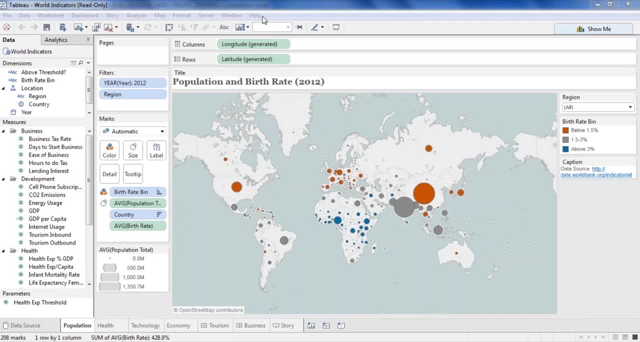 that we can do with Tableau. So it will give you a flavor that we have seen that how we can do a transformation or how we can do ETL, but how we can do a reporting and why we need a visualization. So if you see this, we have some data. 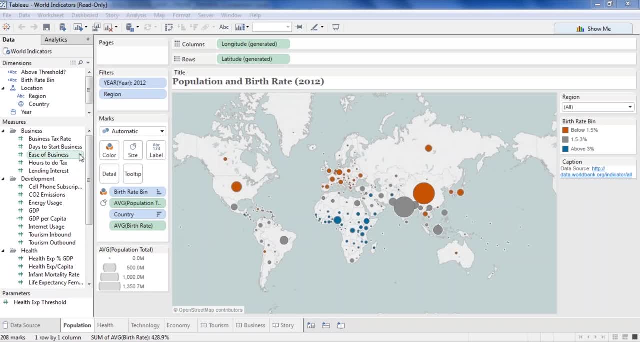 which is known as world data. In this we have something as a region, location. After that we have certain kind of measures. measures that is a factual field. What is the inbound tourism, outbound tourism, GDP, CO2 emissions, cell phone subscription, those kind of things? 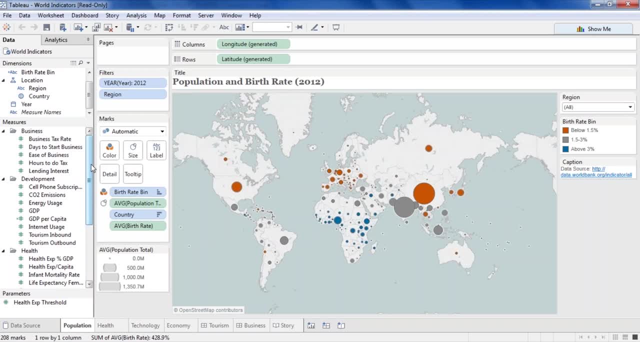 Okay, we have all this data available in our data warehouse. Now I want to utilize that data so that I can make some business decisions. So this is one of the chart that I can create with using Tableau. This is a graph chart, not a location chart. 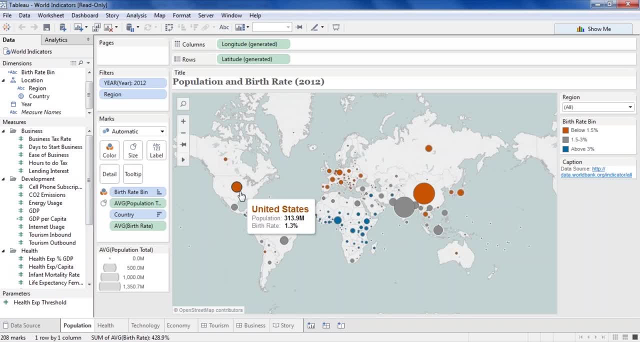 If you can see that. it plots me that: what's the population, how is the birth rate? It also defines me a color. which color signifies that? So if you see over here which is above 1.5% is maroon. 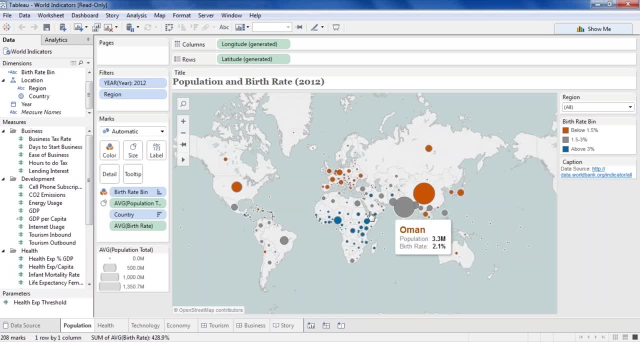 Between 1.5 to 3 is gray Blue is above 3%. Again, with the location it is, with the population, it is a big circle or a small circle, those kind of things. So this gives you a very good visualization. 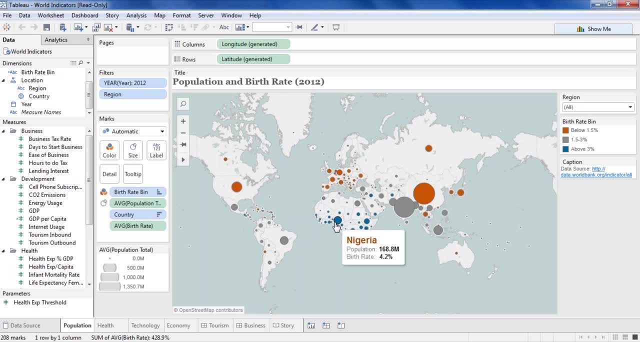 So when you want to present it to your senior managers, you will not be presenting a plain Excel sheet. that okay, this is the Excel sheet. these are the locations, these are the percentages. Now see your data. It will make a lot of difference if you are providing them. 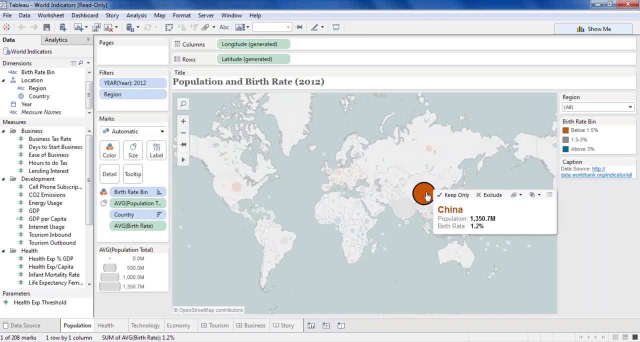 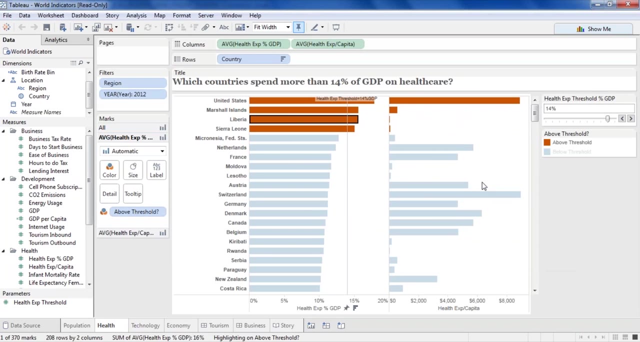 this kind of visualization, That okay, if I click on this, you'll get this, And again I'll get into this more details- that how you can effectively utilize this, or you can create a dashboard out of these reports. So again, you can have this kind of a bar chart. 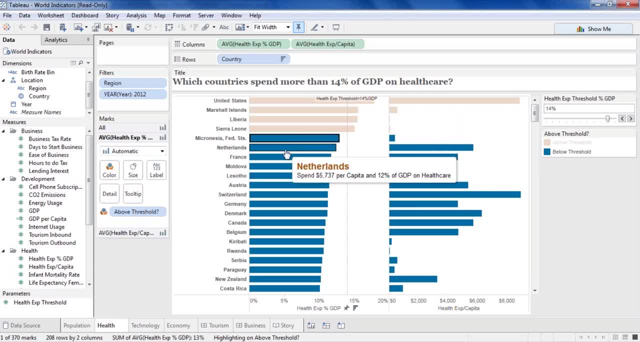 that countries which spend more money on this, countries which spend more than 14% of GDP on the healthcare- again, I can increase or decrease this. I want only 13% as a threshold. I want to increase this as a 15% as a threshold. 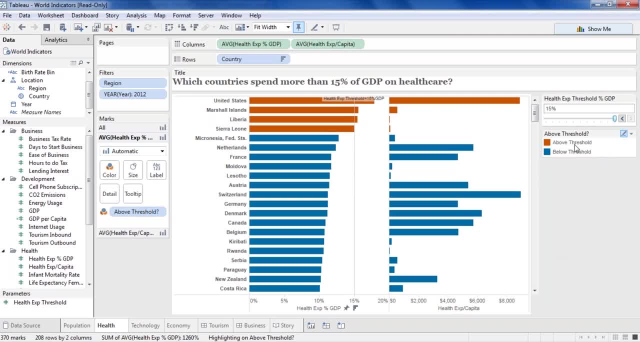 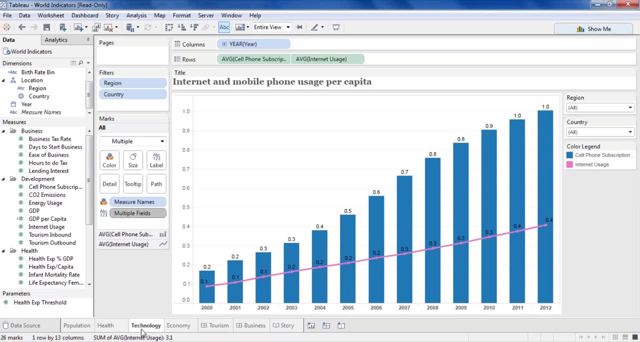 What are above threshold, what are below threshold, Those kind of things or those kind of visual analysis that I can do with the Tableau. Similarly, with the technology, I can create this multiple bar chart, bar chart with a line chart. Okay, again, I can select any region, so that okay. 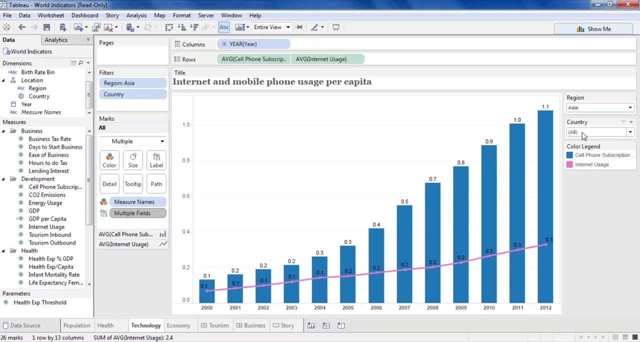 I can select any region so that, okay, I can select any region. so that I can select any region. so that, okay, I can select any region so that it will give me a region-wise thing. Country: there are multiple country. 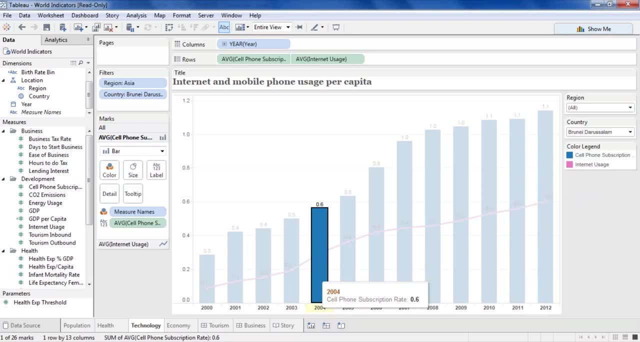 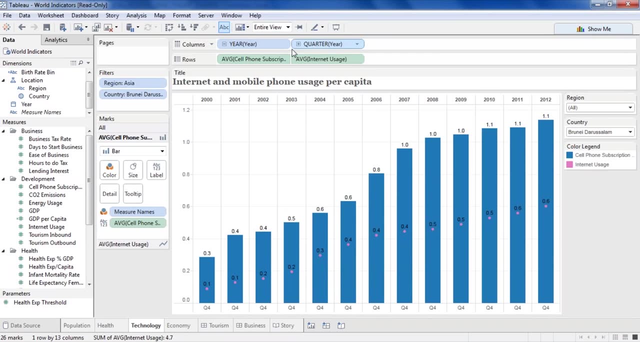 I can drill down to any particular country. Okay, in 2004, I can select this. Okay, so with this year, I can drill down further into the quarters, into the months, that how my data is distributed. Okay, and this, as I am having data only for a particular. 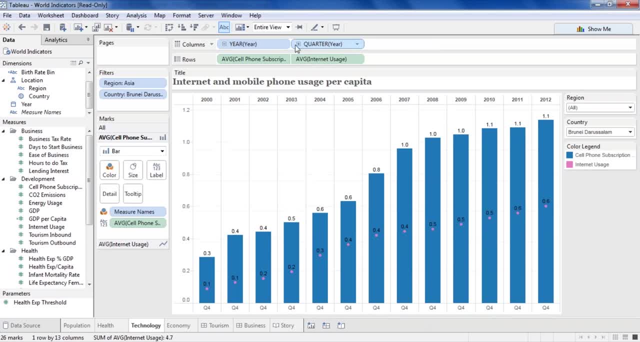 only for a particular year. so there is no point in drill downing. So if you see that every time it is giving me Q4,, So if you see that every time it is giving me Q4, only, but if I had data at the monthly level. 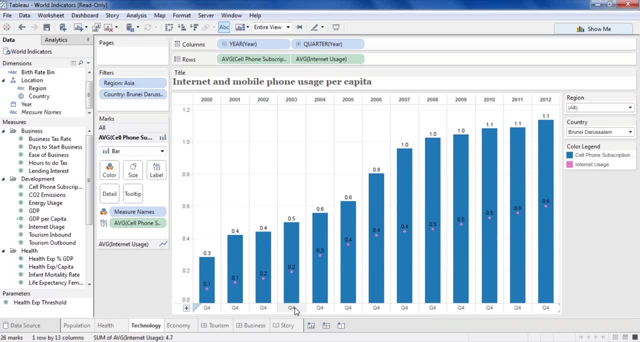 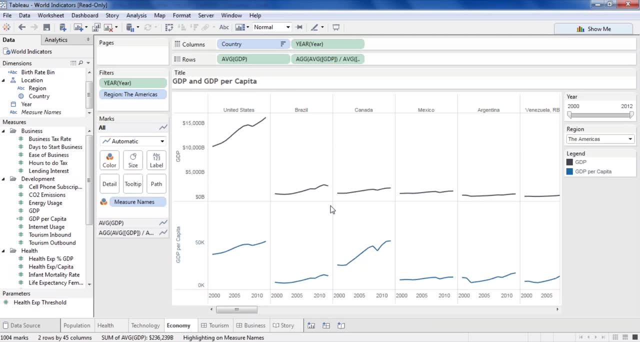 or at the daily level. then I can drill down or drill up and, believe me, it is very fast with the Tableau. Okay. similarly with the economy. I can have this data available with me. that for which duration I want this? 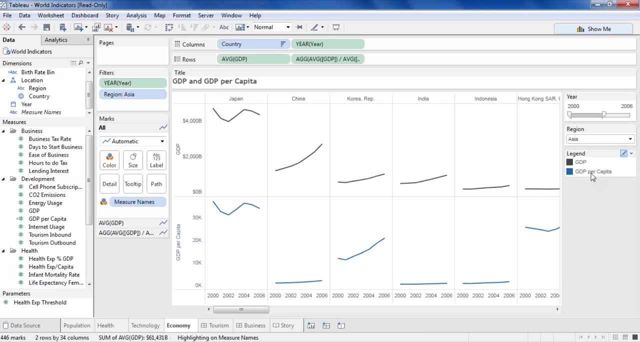 I want this data for which particular region. Each line will show different thing: that it is GDP per capita GDP. I want only China, I can keep only, and those kind of things. Okay, there are a couple of questions here. 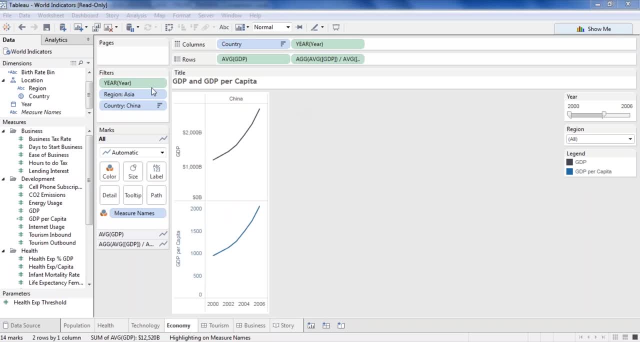 What are the major concept or the major part of BI and what are the programming knowledge required? Any coding is required for Tableau. No, so there is no knowledge, no coding knowledge or a programming knowledge required for learning any of the tools. may it be Tableau, may it be talent. 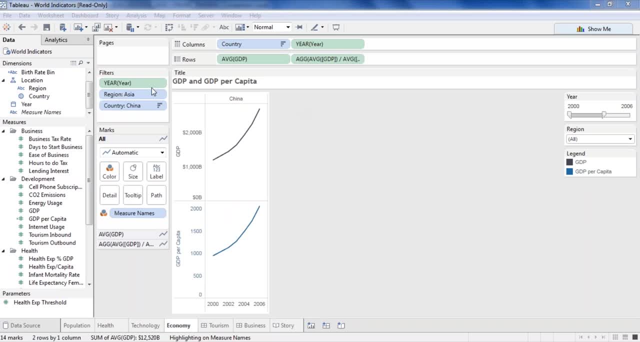 So that is the best part of the talent. There was a question earlier with that- how big data integrate or how can I integrate with them, or how a group integrate with the talent, And the reason why these tools are available is that you don't need to have 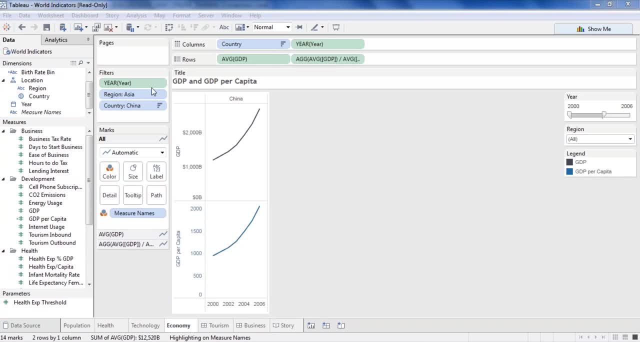 an in-depth knowledge of the programming, Even if you have basic knowledge or no knowledge. you just need to have your concept right that what you want to do with the BI, what kind of data that you want. So maybe this kind of Tableau reports. 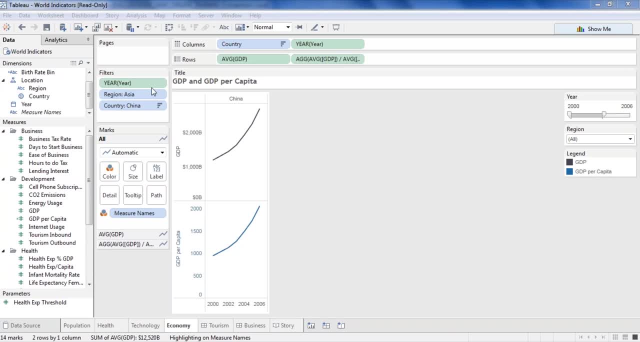 if there is an analyst- maybe a finance analyst or maybe a report analyst- who is not at all into a programming knowledge, if you give him or her the data, they can create their own visualization so that they can present it well. So it is not at all needed that you need to learn. 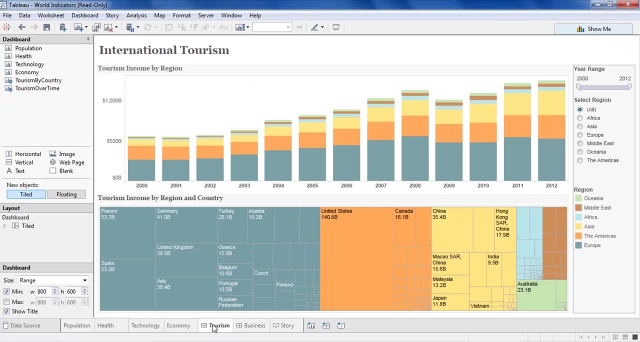 certain kind of programming language or certain thing beforehand. Okay, coming to this, this is known as Dashboard, where we have multiple reports into a single view. So I want to see this. if you see this Dashboard, sorry. Tourism Income by Region. 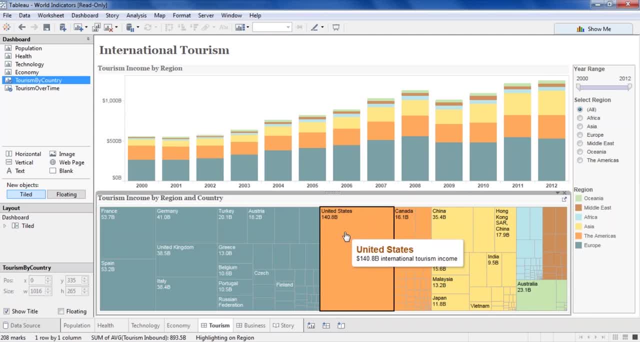 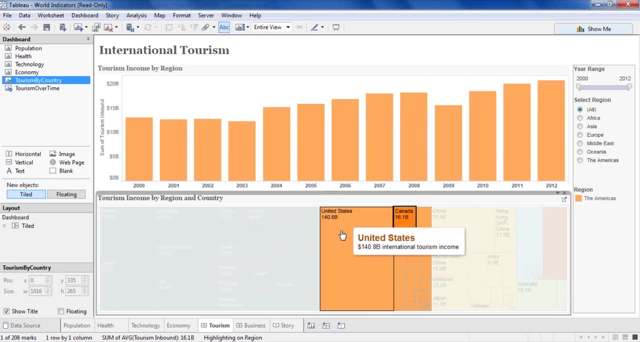 Tourism Income by Region and Country, those kind of information. So if I select on one particular thing, you can see that that particular chart is highlighted. If I select on this particular, this channel chart is highlighted. I can again change this thing. 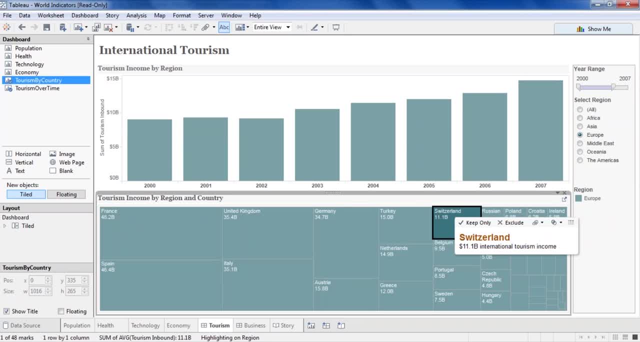 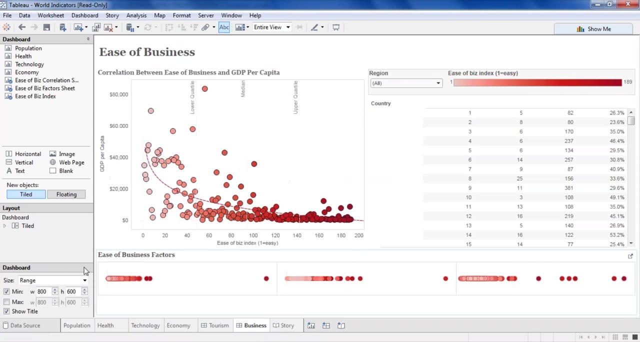 I can go only to Europe, and after that again I want to go into this particular Switzerland. So there's some of Tourism Income is only for Switzerland, Okay, so this way, this kind of interactivity Tableau provides you Similarly with the Business. 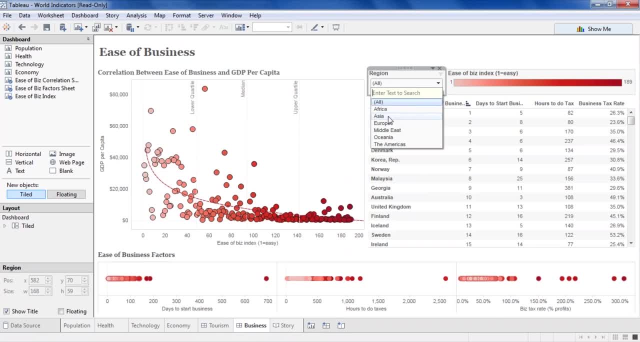 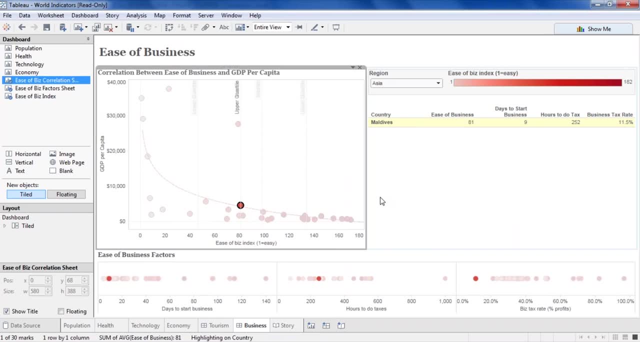 I can select on any one particular thing: Particular region, maybe for Asia, I want to select Hong Kong, or I want to select this particular Maldives. I will get data only for Maldives. Ease of Business Factor. what's the ease of business? 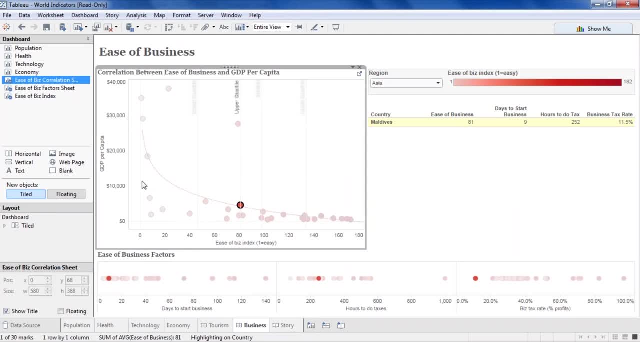 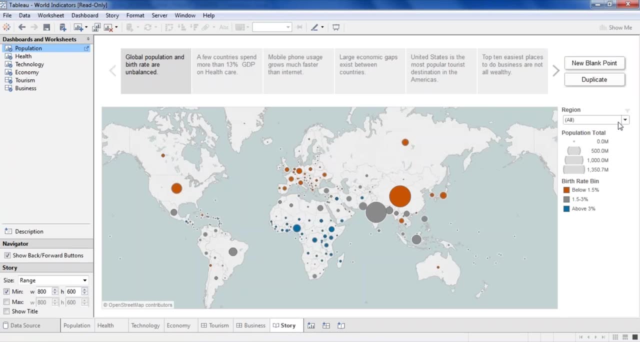 business rate, percentage, profit, everything. So this is how you can use your BI tool. So, with the Story, if you see that it will get you, and if it will get you, then you need to set it up for a new BI. 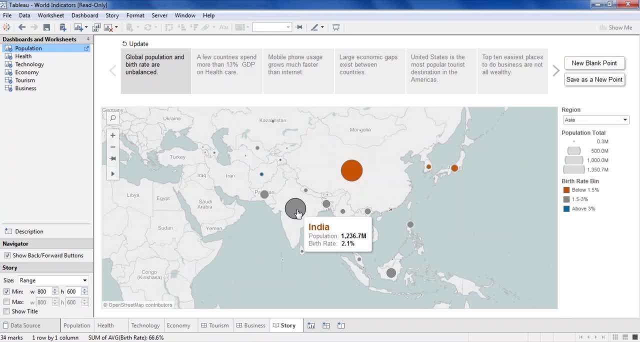 Similarly with the Story. if you see that, it will get you you a detail that, okay, where the population is more, with the big, uh, with the big circle or the small circle and the color indicating that. so that is, that is it, or that is how this tableau works. 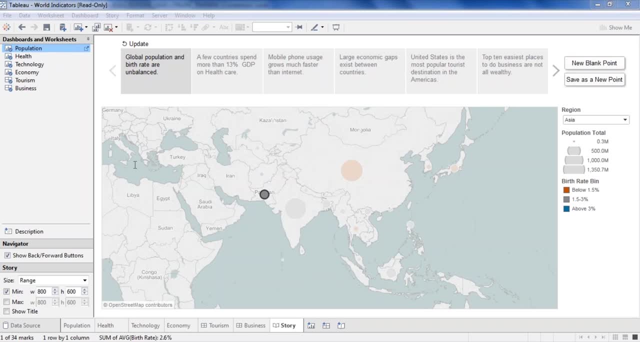 for the bi purposes and you can see with this, with the visualizations, right, uh, we are. we are already three minutes over, uh, over, but still, if you have any questions, uh, i'm ready to answer that. uh, so quickly. if you have any questions, uh, we can cover that up. let's, we can close that.